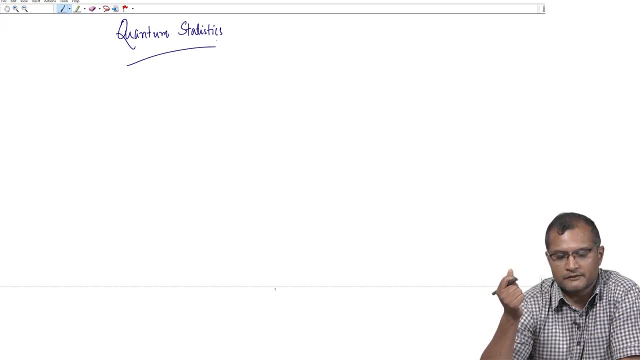 question that arises in our mind is that: why do we need a different level of statistics for quantum systems? Now, to understand that, we must first identify what is the quantum limit of any classical system, or what is the classical limit of any quantum system, That 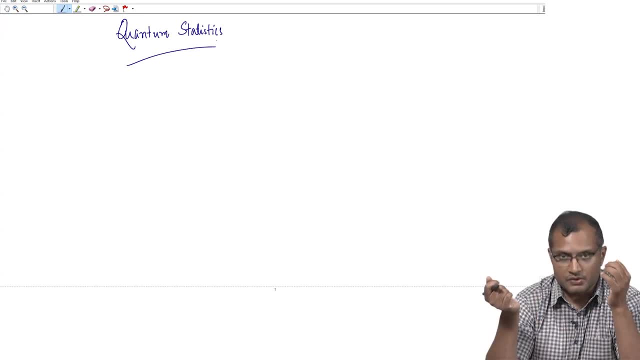 being said. Now, looking at the same system, the system does not change, but it may so happen that, for a combination of temperature and density, the system at our disposal may behave quantum mechanically, Meaning that it is no longer representable by a deterministic set of rules. 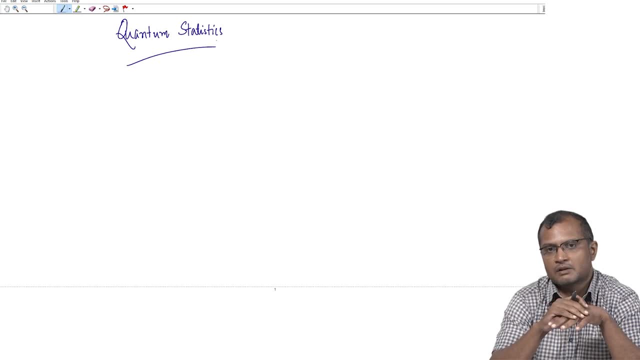 which means at some sufficiently high density or sufficiently low temperature. I will discuss in a short while what do we mean by sufficiently high or low. So at high density and low temperature you would replace classical mechanics with quantum mechanics, and we have already seen some kind of a discussion on the onset of quantum mechanics in classical 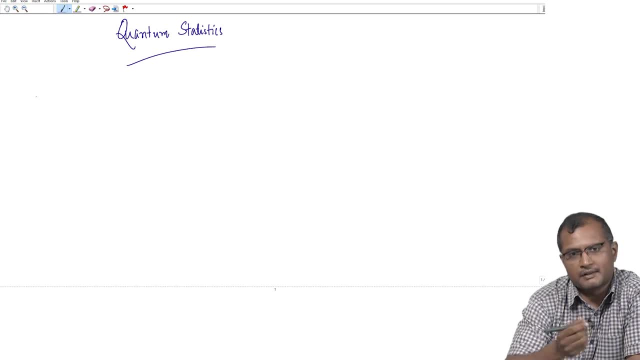 systems, with a small recollection of the fact that. So first, before we recollect anything, I would like to put down the points in some order, just figuratively, to basically decide what we are going to discuss. ok, So the first thing on the cards is basically: 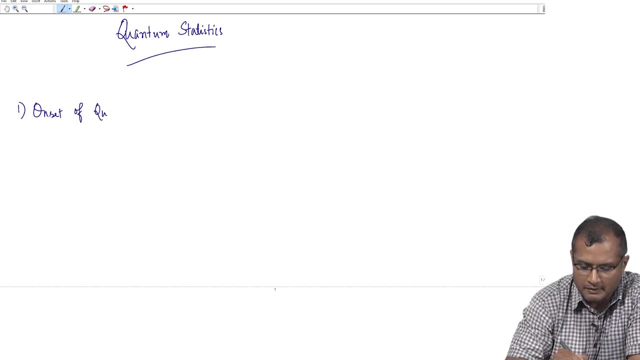 concept of quantum mechanics. So when should I be worrying about quantum mechanical effects As the first thing to ask? because otherwise, after chapter 1 and chapter 2, I know exactly what to do when somebody asks me to compute the heat capacity of a material or susceptibility. 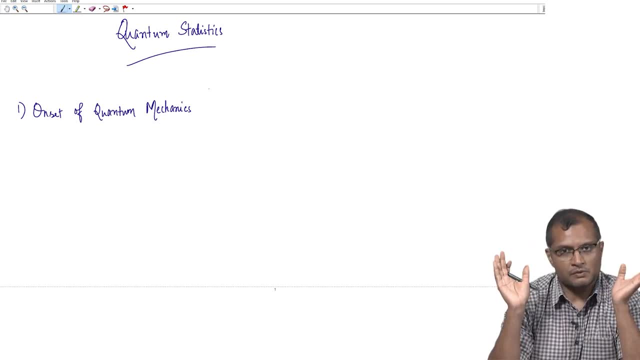 of a magnetic system. All these questions can be answered using tools of classical statistical mechanics. But the same system at my hand, for example, electrons in a metal or spins on a lattice- will classical theories suffice? will they give me the right answer? The answer to this? 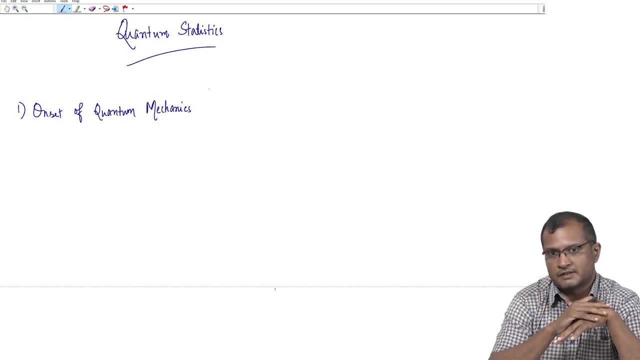 question relies on the physical parameters of the system, which are the density and the temperature that should decide whether I am in the quantum regime or classical regime. we will discuss those parameters very shortly. The second point in this chapter would be basically a machinery or a theoretical set of tools that appropriately handles the system of indistinguishable 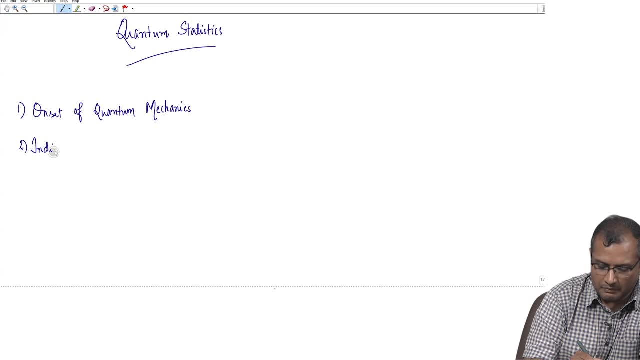 particles. Now, you have seen, in classical statistical mechanics, we do not know how to handle these indistinguishable particles, except for the fact that once you complete a calculation, you account for the fact that might be the microstates which are only different from each other in only permutation of identical 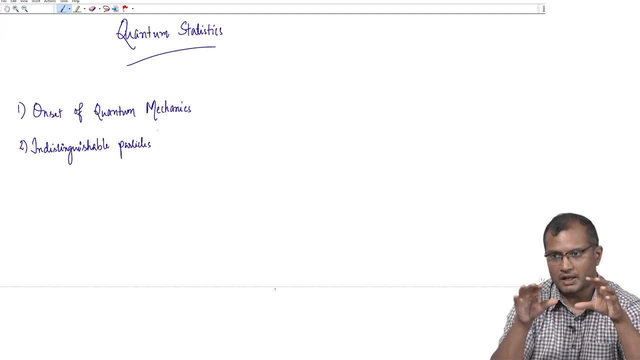 particles are to be seen as just one entity, And so you in some sense plug the n factorial pre factor after you have completed your calculation. There is no inbuilt machinery in classical mechanics which handles indistinguishability of particles, So we will see how quantum 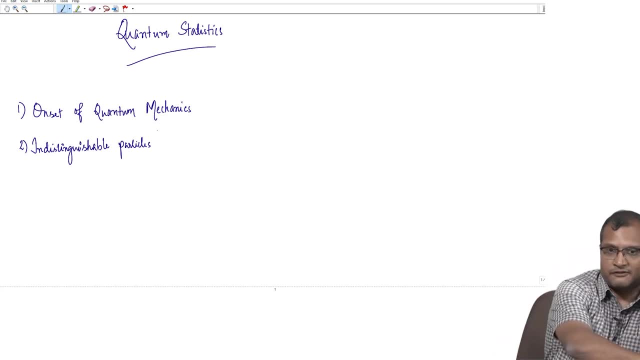 mechanically, you know, starts off. So, with this correct formalism, as if it is embedded in its DNA. ok, So the n factorial is not going to be missed. it, in fact, it will be plugged into your calculations from the beginning itself. that is number 1.. So, in the context of indistinguishable particles, 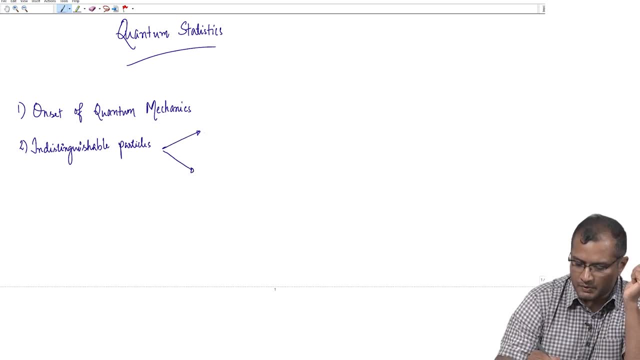 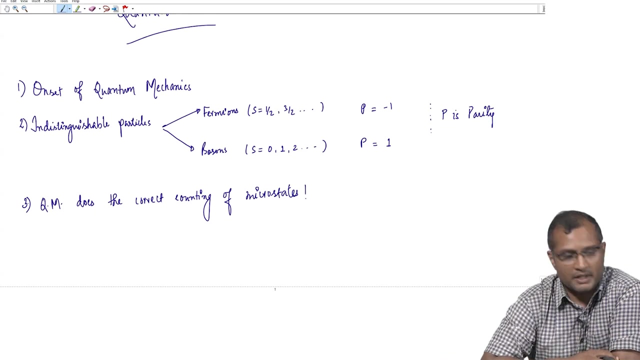 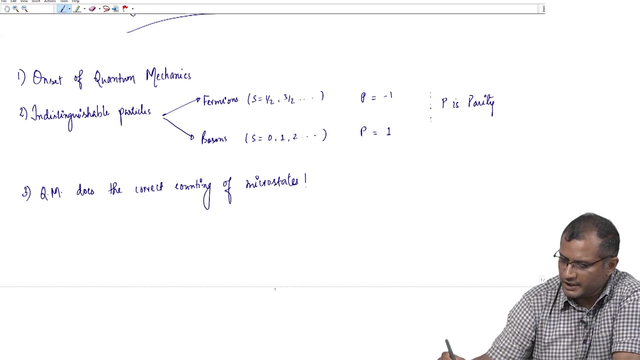 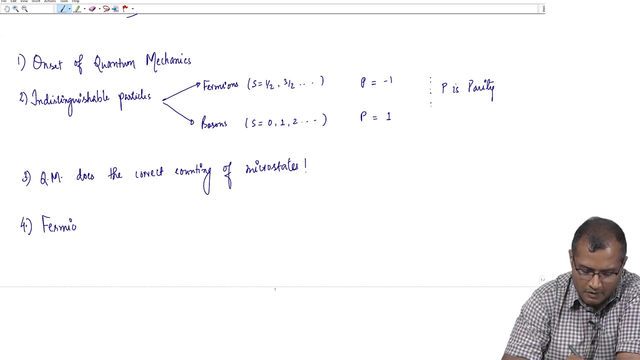 we will be discussing two types of particles, which are fermions and bosons. Actually, there is a previous countermechanism and there is an interesting looking countermechanism above all other metaphysicals. It is also quite similar because Radenshitz, with itsört ranging from 0 to 4000, point zero bound. yeah right, that number solamente goes from 0 to 100, point 0 to 1000.. And in those courses, bottom of the chart. 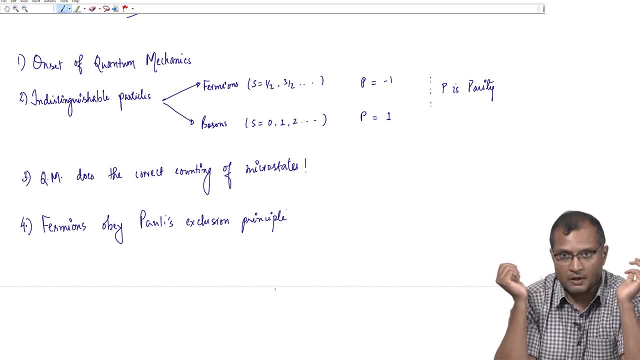 So one you can explain why this 5200 is not going to be gone. You can just imagine the four energies going together and if you imagine one of these methods by using the two punctualetched arrays in some form, So these are all put into the four Color. 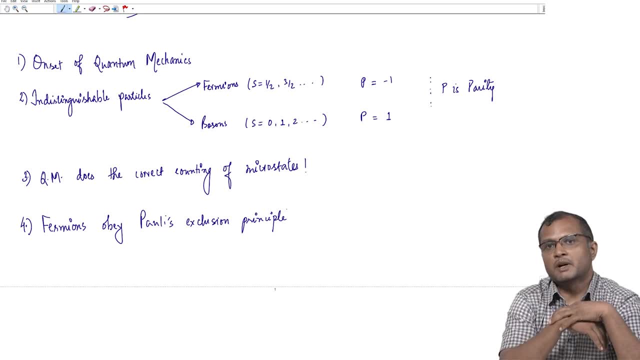 No 2 fermions can exist in the same single particle quantum state. because if you try to force 2 fermions in the same single particle quantum state, then the entire wave function of n particle system will collapse to 0. When you say that the wave function is collapsed to 0, you mean to you are saying that explicitly. 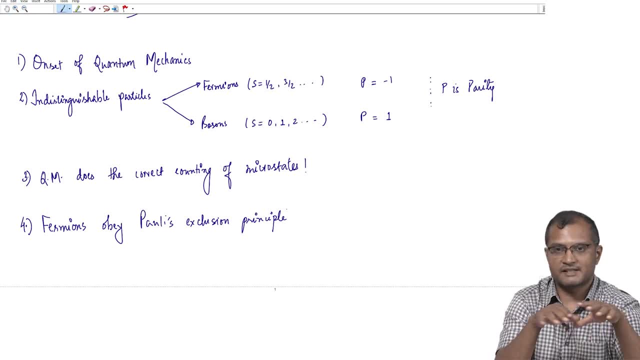 that microstate has 0 probability. so you will never see this. So that is the sort of a sketch or the bird's eye view of what I am going to present in today's lecture. So let us start with the first point on the menu, which is onset of quantum mechanics. 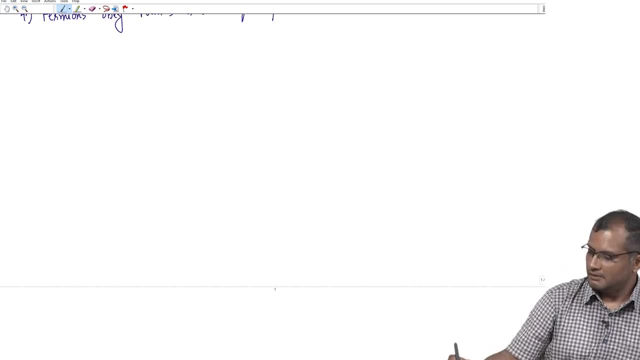 Now we have seen in the second chapter that. So if the temperature is too low, the temperature is, the length scale will vary. You can call it de Broglie wavelength or de Broglie length scale, whatever comes to your mind. that is not necessary, but its form was. we had discovered that this length scale is: 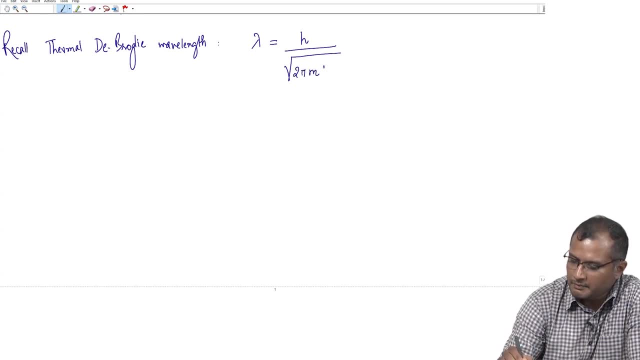 the Planck's constant, h over 2 pi m, k B, T, where k B is the Boltzmann constant and T is the temperature of a system, h being the Planck's constant. Now, I had said that every system that you study, let us say n particles in a box, or electrons, 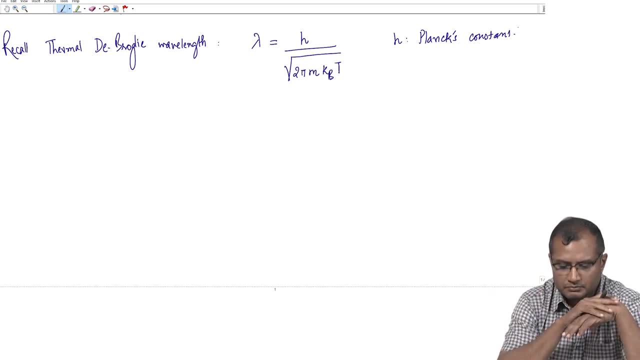 in a metal or gas in this room. you have a certain container or you have a certain box where your particles are. you know they exist. So I know that my system has a density. I call it as small n number density, which is the number of particles in the system over the systems volume. ok. 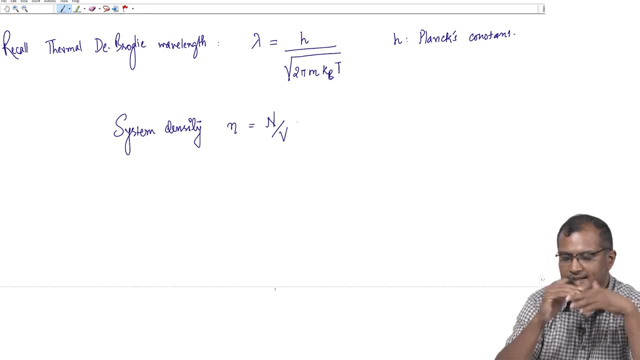 So now you can see that this density has the units of. you know it has the units of just L to the power, minus 3 because of volume. Now, like I said in the beginning few lectures ago that if you want to see the nature of 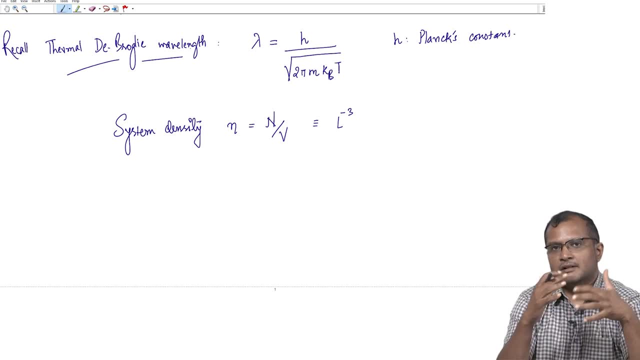 the system. we can always construct a few interesting dimensionless numbers that will tell us how my system will behave. ok, So with one length scale, lambda, I am going to construct another length scale from my density and compare these two length scales by constructing a dimensionless number. 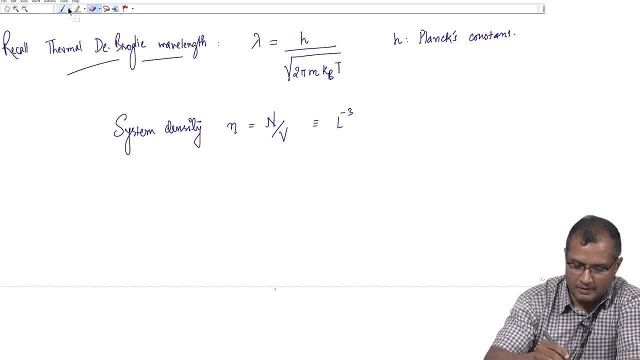 So straight forwardly, I can construct one dimensionless number, construct a dimensionless number, ok, You are free to construct other numbers also. by the way, you can also construct another. So you can take lambda as one length scale, our de Broglie length scale, you divide it. 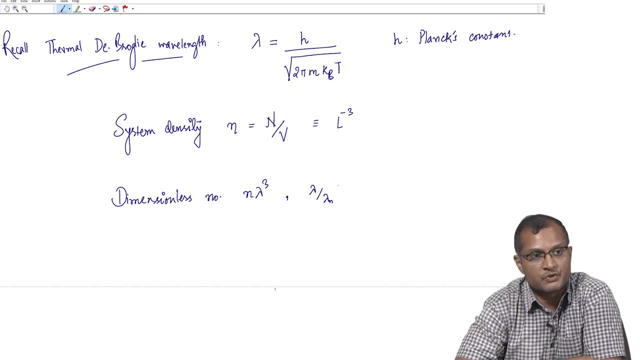 by some density dependent length scale. this is another dimensionless number. Now, how do I construct this lambda n? This lambda n is, you know it can be taken as some n to the power minus 1 by 3, but since we normally work with density, which is known to us, for example for copper, I know that 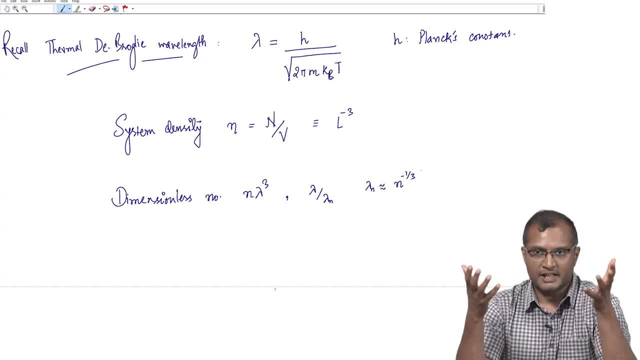 the number of electrons in the metal- So 3 electrons- is of the order of 10 to the power, 28 per meter cube. I know the densities, I know the density of hydrogen in this room, So I would like to work with this combination of you know this dimensionless number where? 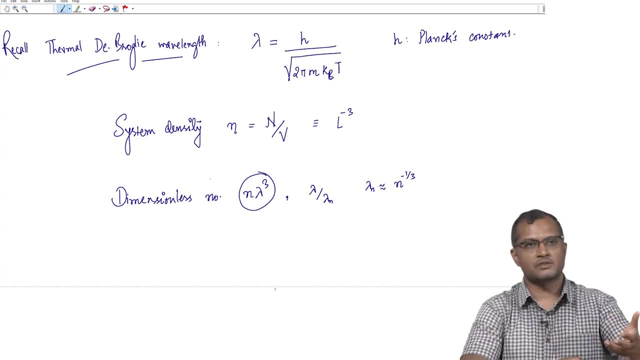 I know n you know from handbook of materials or by previous laboratory experience or whatever, and I know to very good extent what is my de Broglie wavelength. So you can choose to work with this dimensionless number purely for convenience sake. 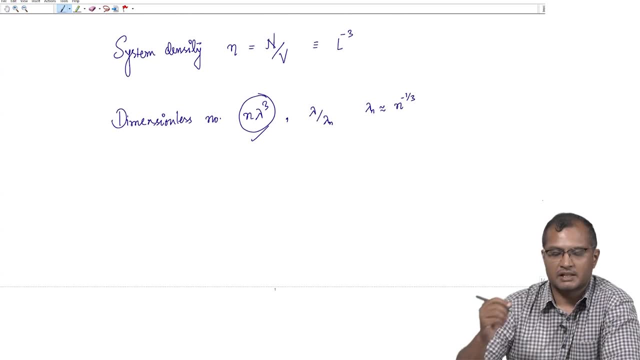 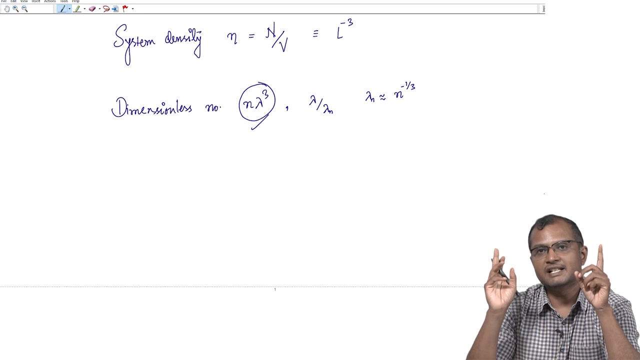 So let us pick up this dimensionless number and see whether we can distinguish the 2 worlds, quantum and classical. So clearly. I know that the limit of high density and low temperature is the quantum mechanical world, because this is where, when you take, when you look at the expression for the de Broglie, 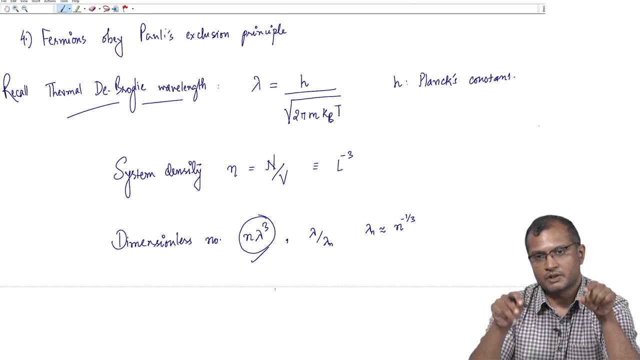 wavelength. this wavelength will be very large at very low temperatures. as the temperature goes to 0, lambda goes to infinity. So the wave nature of the particles becomes to dominate. it becomes essentially more and more delocalized. So I know that for low temperature is the 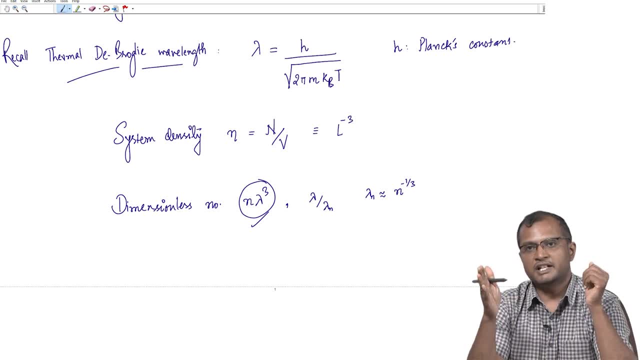 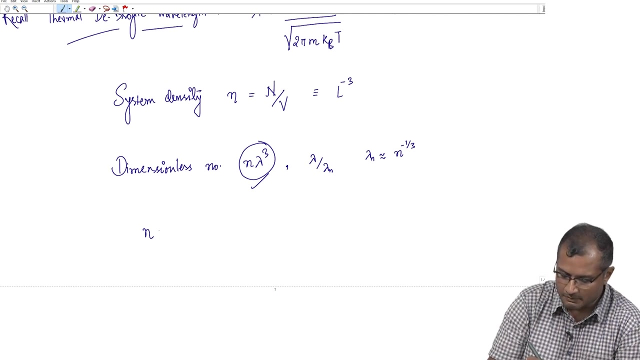 quantum regime. I also know that if I for any temperature, I can increase my density, thereby making the inter particle separation smaller and smaller, in such a way that this separation can be made smaller than the de Broglie wavelength. that is also a quantum limit for my system. So one thing is clear: that the dimensionless 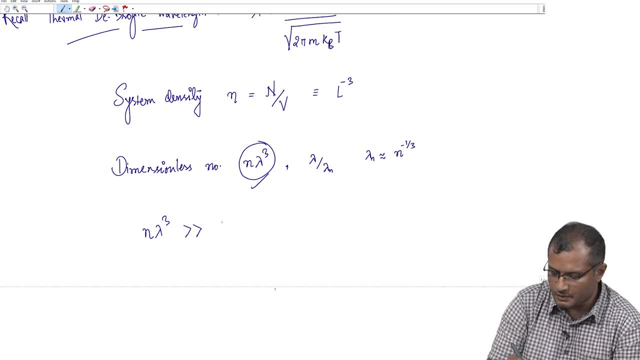 number n, lambda cube being much larger than 1. is the quantum regime? Ok, The regime where I make both n and lambda larger and larger? ok, because lambda is large means my wavelength is getting large. my wave nature of the particles becomes more and more. 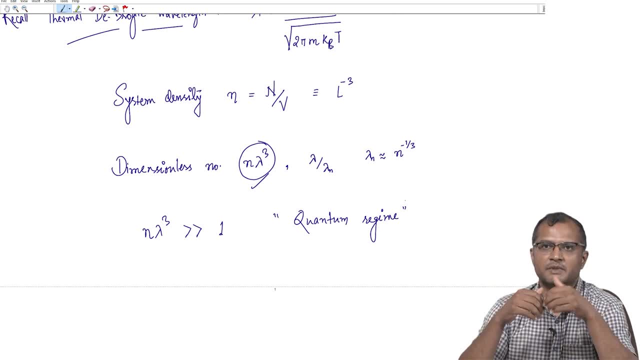 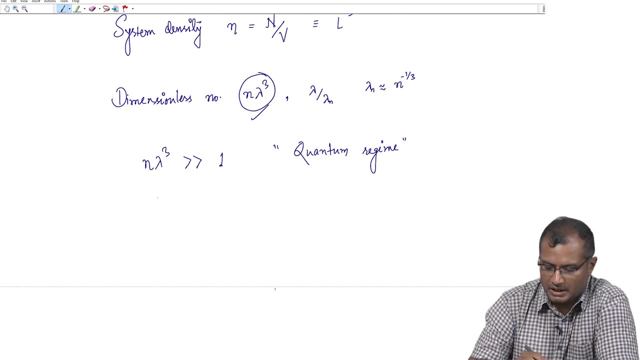 predominant. and density being large means my inter particle separation is also much smaller than the de Broglie wavelength. So this is definitely a quantum regime. ok, So I will show by calculating numbers. this is definitely quantum regime. I also know that. well, just by the preceding argument we can push this limit to the other side. So I can. 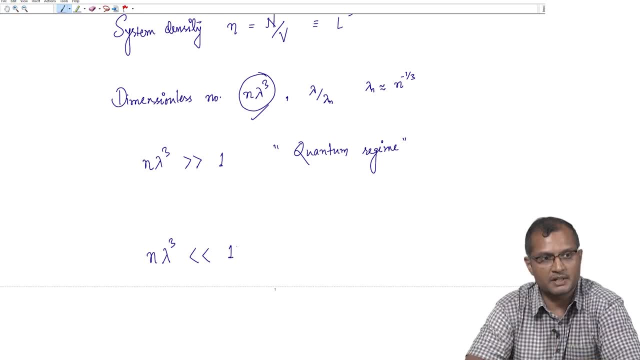 say that if this dimensionless number is much smaller than 1, ok, then I am in the classical regime, Ok, Ok. Ok, Of course, because I can push n lambda cube to be much less than 1 by making n very very. 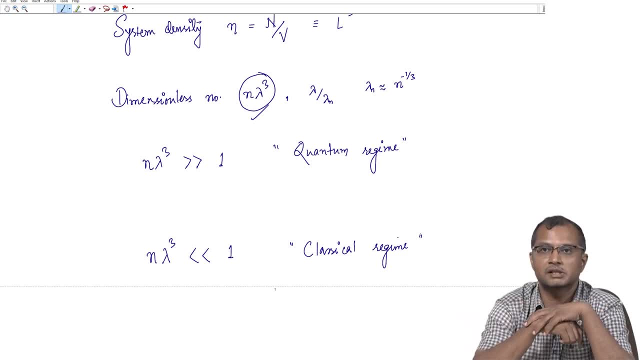 small, thereby increasing the separation between particles, such that the particle separation far exceeds the de Broglie wavelength. ok, And lambda is also being very, very, you know, is made very small, which is like increasing temperature, because lambda is proportional to 1 upon square root t, So both n and lambda are increased. that increases n, lambda cube. 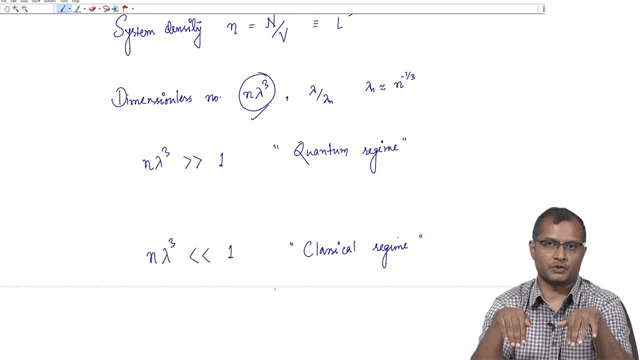 and both n and lambda are reduced. that reduces n lambda cube. It is very simple to see why one leads to a quantum effect, the other leads to a classical behaviour. Naturally, there is a boundary that separate these two and the boundary is not sharp. the boundary is 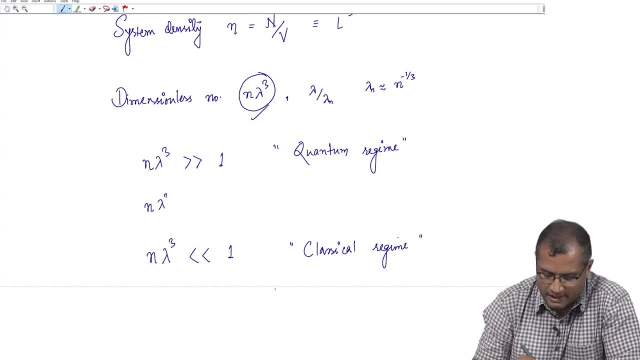 fuzzy. ok, And I will say that n lambda cube of the order 1 is the onset of quantum mechanics. Ok, This is where you will sort of say that I am not very clear which theory will work, but I am sure that the quantum effects are not ignorable and n lambda cube is of the 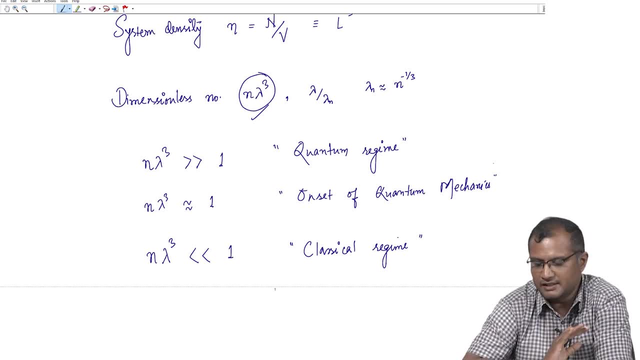 order 1.. It is tricky, it is not easy. It is very safe to handle the two extreme regimes where the regime n lambda cube, being much smaller than 1. Almost guarantees that your classical calculations will work with you know they will come out. 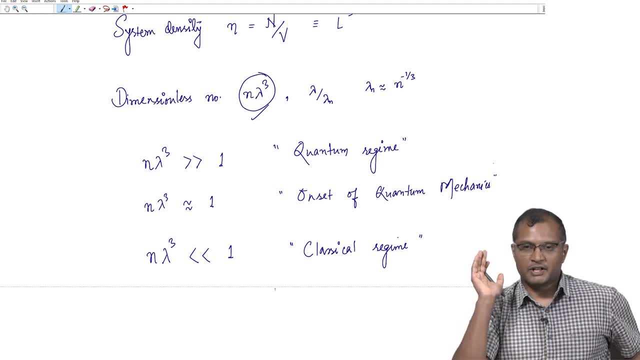 with flying colours. In the regime n lambda cube greater than 1, classical theories will fail miserably. And this is the regime. where you have, you know, electrons in a metal, you must invoke a quantum calculation. ok, For electrons in a metal at room temperature: 300. 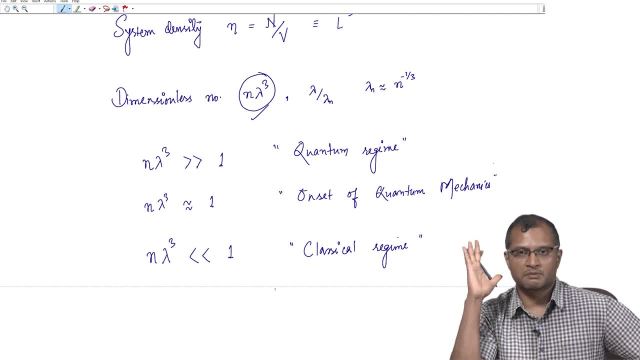 kelvin, you will very soon calculate that n lambda cube is much larger than 1.. you must invoke a quantum calculation. All your Debye, your Dulong-Pettit law, will fail miserably for heat capacity of a metal due to electrons And when this dimension is number. 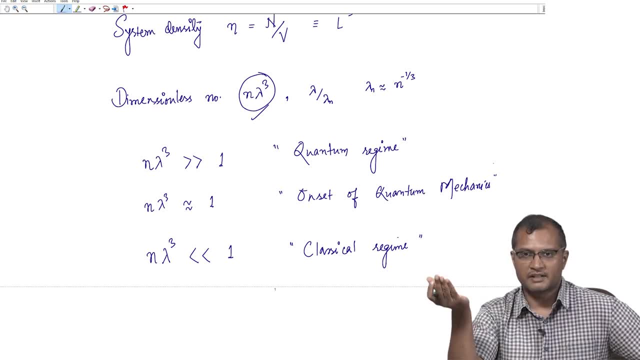 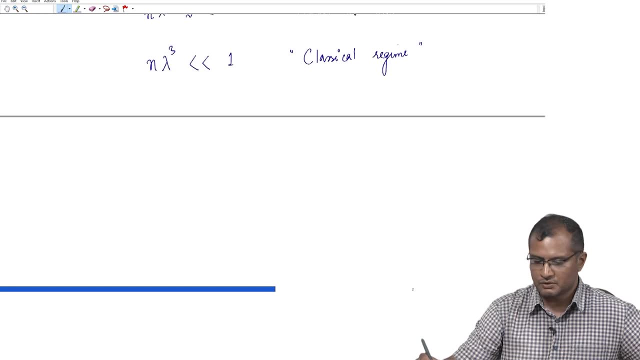 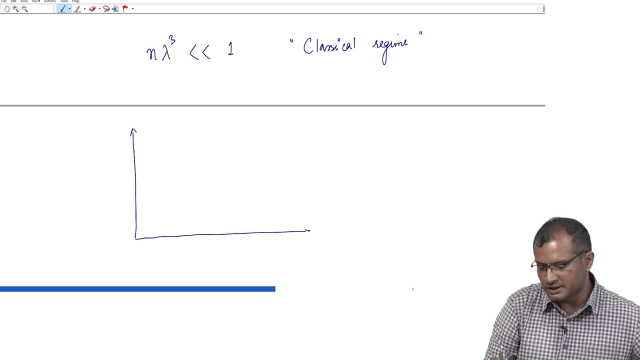 is of the order 1, you know that you have to be careful, because this is the regime when quantum mechanics begins to show its presence. So then you can actually construct some sort of a parameter space, space diagram where, at least figuratively, you can say whether 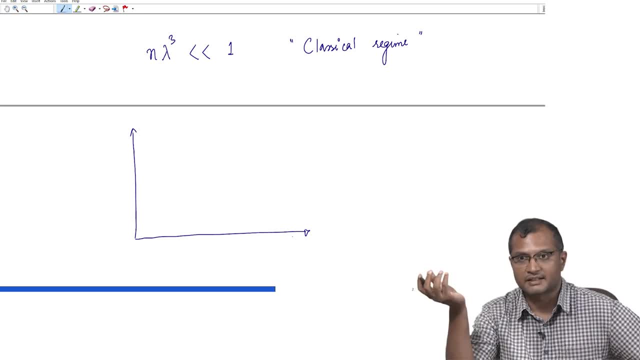 quantum mechanics is applies, or quantum mechanics or classical mechanics applies. So you can say that I will construct a T-N diagram, number density versus temperature and show, in which you know, the region of applicability of classical or quantum mechanics. Clearly there is a line. 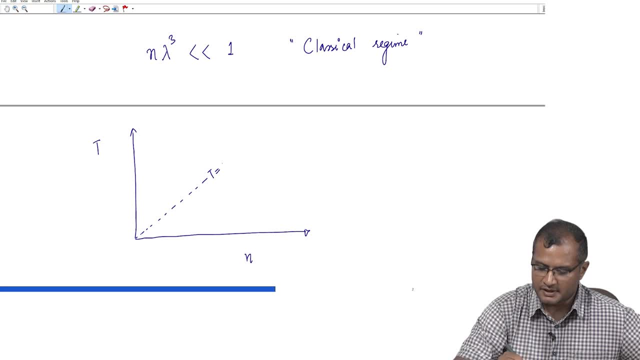 of The line of 45 degree slope, which is the T equal to N curve, and my curve, N lambda cube equals to 1, would be somewhere like this. So this is my curve, So deep inside this phase. so this curve that I have computed, the solid line is the. 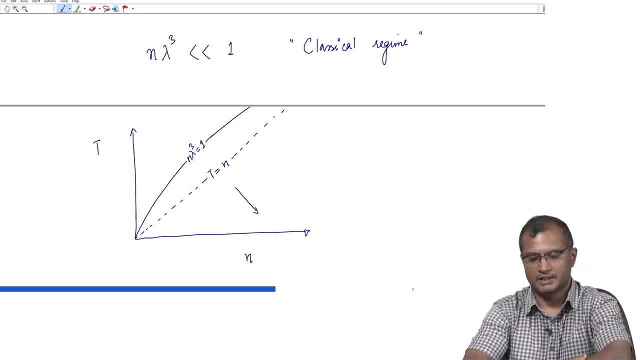 line of N lambda cube equal to 1, and deep inside this phase, you will say that your system has quantum effects, Because that is the region Where the, Where the, when you have high density and low temperature. and deep above this solid line, you will say: 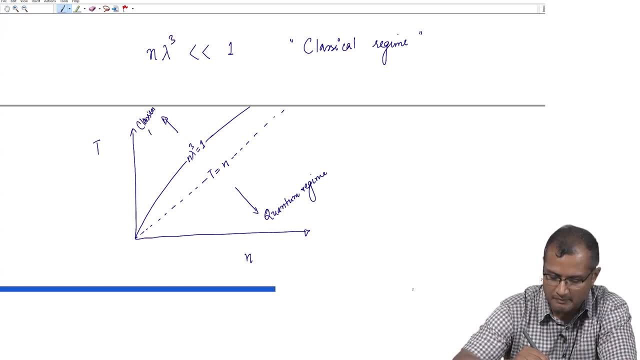 that I have a classical regime. ok, And somewhere close to the n lambda cube equal to 1 line, you have a- you know, onset of quantum mechanics. So I will say I am going to remove the t equal to n line because it is making the figure very busy. just maybe very faintly I will show. 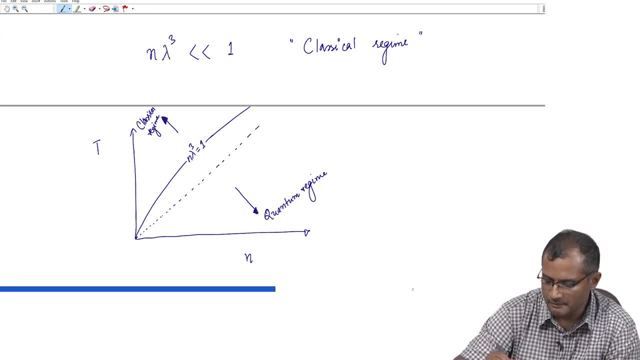 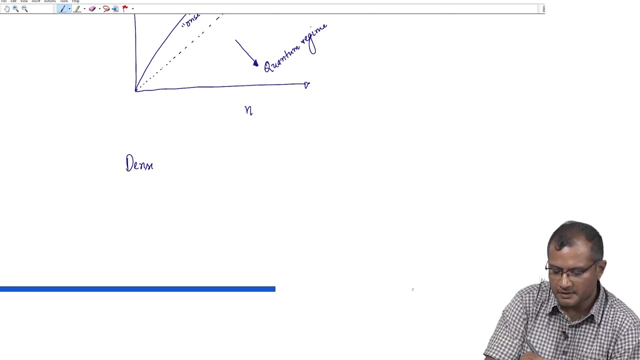 ok, So this is where I have the onset of quantum mechanics near the solid line, Just to give you a feeling in terms of numbers. So if I compute the, I will say: that said, what temperatures do I see? quantum mechanics, See, that is the question. 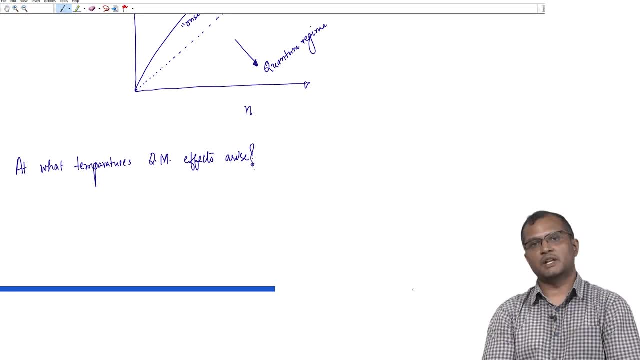 at what temperatures the quantum mechanics begins to take over. Well, you have this relationship. So if that is your question, you can answer this by saying: this is the fuzzy boundary: n lambda cube equals to 1.. This will give me the temperature when quantum effects will. 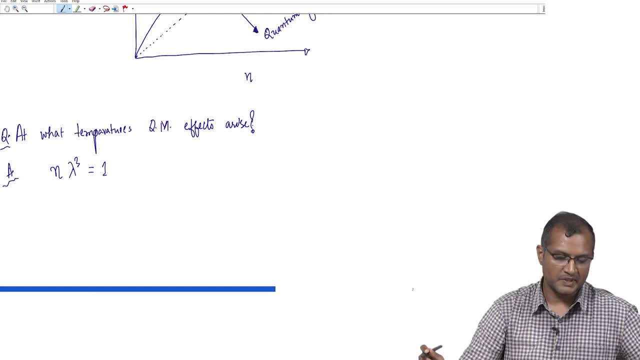 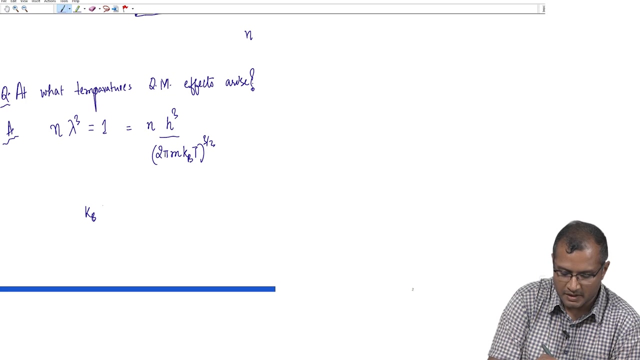 begin to, you know, take effects, And I know this is nothing but n times H, cube over 2 pi m, k B T to the power 3 half, because that is the definition of lambda. So now you can compute the temperature from here. So you can say that my k B T and this: 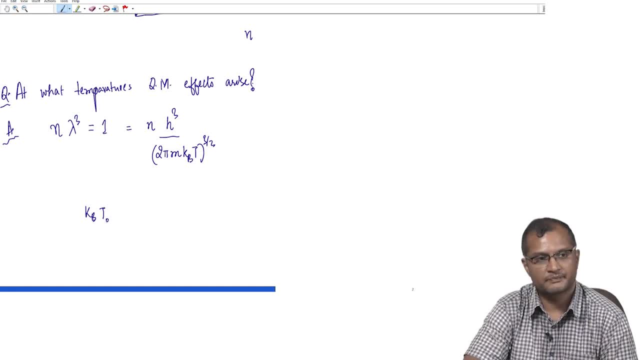 is nothing but the, in some sense the degeneracy temperature where this particular T is when n lambda cube is 1.. So I am just calling it as T naught. So if I take k T on the other side I will get k T to the power 3 half as n times h cut. 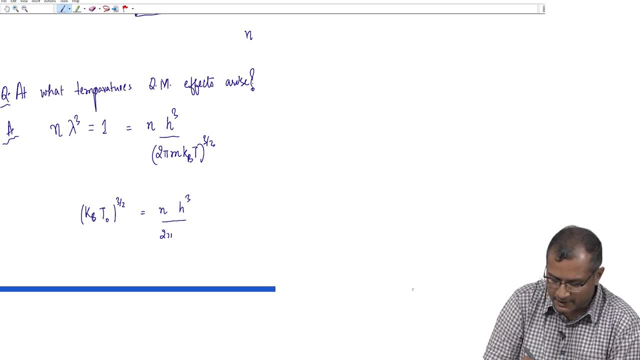 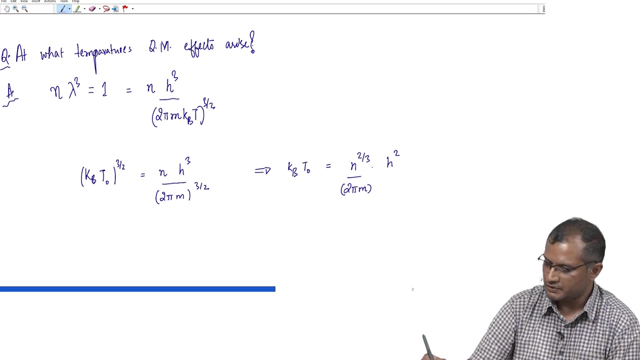 h cube over 2 pi m to the power 3 half. fine, Just multiplied both sides with k T to the power 3 half, And this gives me k T as nothing but n to the power 2 by 3 into h square over 2 pi m. and naturally, if you compute, So if you just 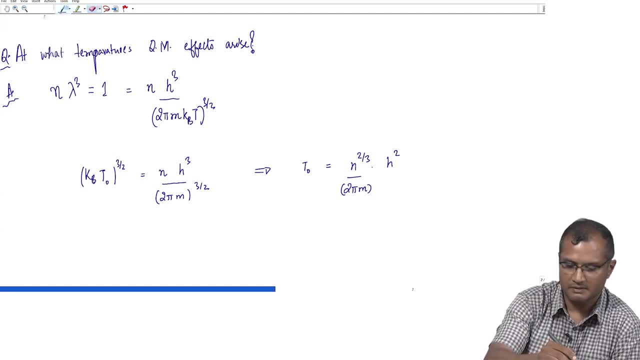 you can write down this. you can divide it by k, B on both sides. So this is the, basically the temperature that corresponds to your n lambda cube equal to 1.. So this is the temperature at which quantum mechanics will begin to take effect. Let us 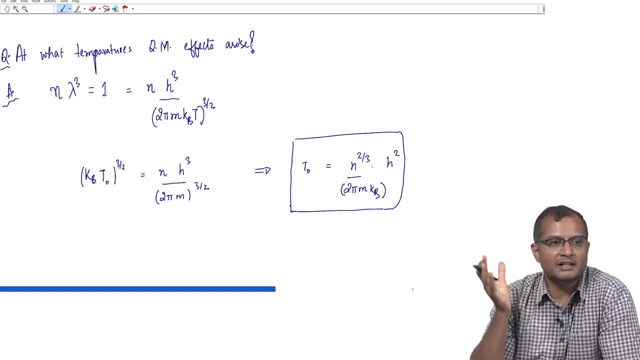 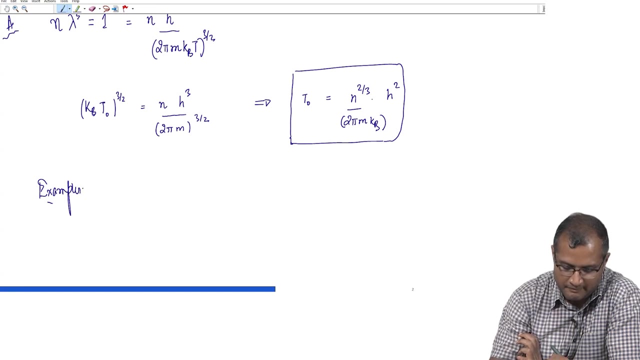 compute these temperatures for some of the systems that we routinely encounter in our everyday lives. It will give you an idea. you will appreciate the fact. Why should I learn quantum mechanics Right? So I am going to take some examples. The first example that I am going to take is that of a, you know, hydrogen. 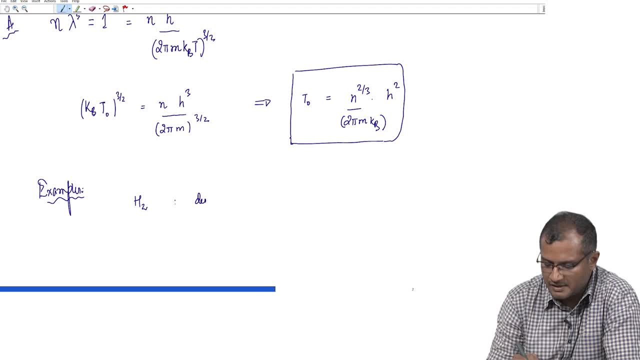 So hydrogen, for instance, has a density and I have written it down here: has a number, density of 2 into 10 to the power, 19 per centimeter cube. So this is the number density for nitrogen. ok, So this is the N for nitrogen. 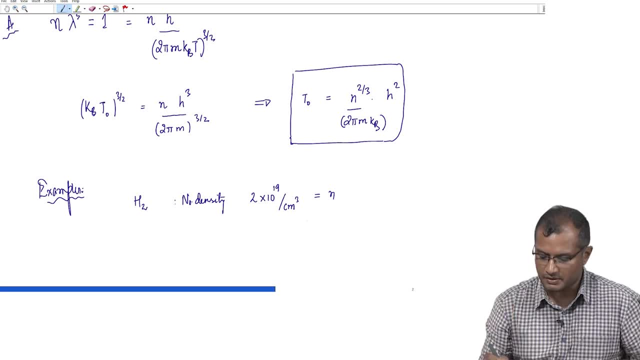 Now, if I want to compute the degeneracy temperature, so this gives me the degeneracy temperature here. If I compute this, it comes out to be around 5 into 10 to the power minus 2 Kelvin, So somewhere around 0.05 Kelvin for hydrogen. you must invoke quantum mechanics or you must. 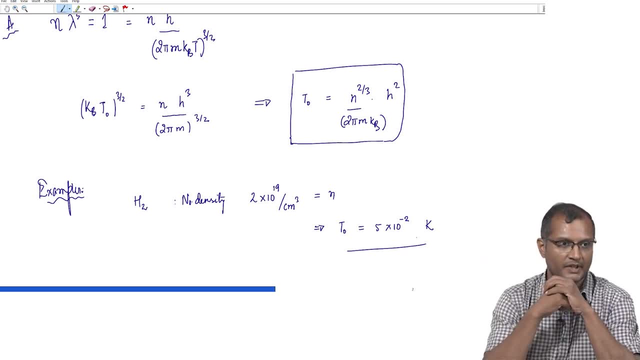 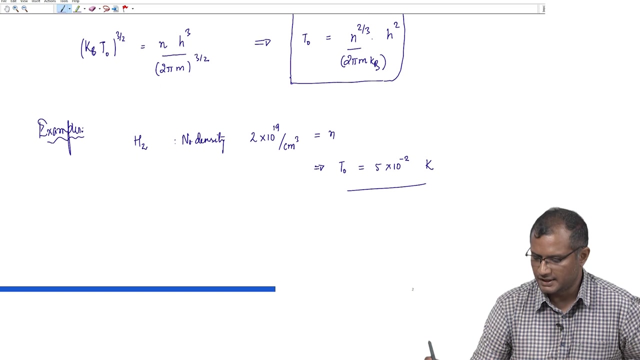 invoke quantum statistical mechanics. The classical calculation is perfectly valid at room temperature, Only at this low temperature. your N lambda cube is of the order 1, that is the meaning of this calculation. ok, Let us take another. is there a question? 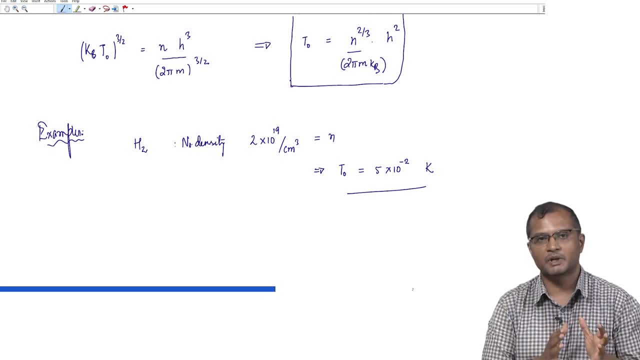 Which tells you what See? I computed this temperature by equating N lambda cube as 1, which is the onset of quantum mechanics. At this temperature you will see quantum mechanical effects. Higher temperatures, definitely. I will be classical, ok. So unless you push your temperatures down to 5, into 10, to the power minus 2 Kelvin which 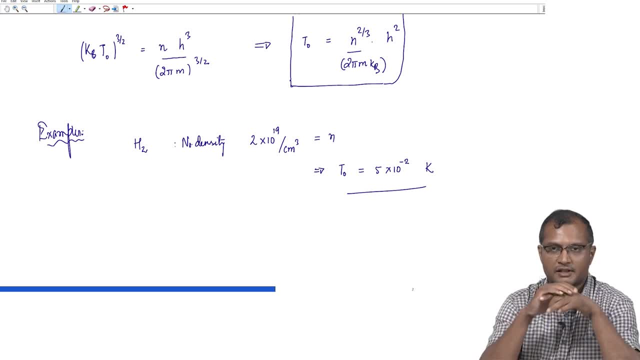 is like 0.05 Kelvin. you can treat hydrogen in the air classically. Let us take another system, which is helium 4, liquid helium. ok, So this has a number density of. So this density of liquid helium has a number density of 2 into 10, to the power, 22 per centimeter. 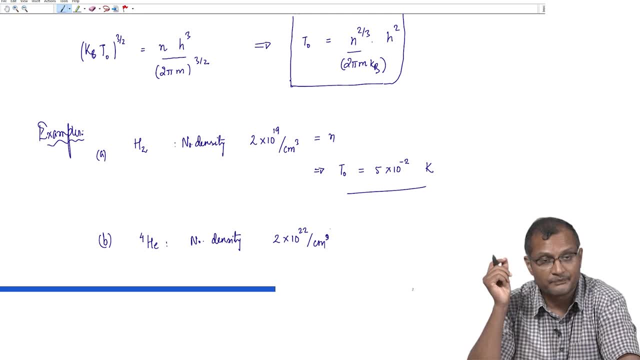 cube. Now this is a higher density, So I can expect that the degeneracy temperature will be higher, because now I should see quantum mechanics effects at even higher temperature. but this guy is already sitting at a higher density. ok, So this is the N for it and you plug this number density in the in this expression that 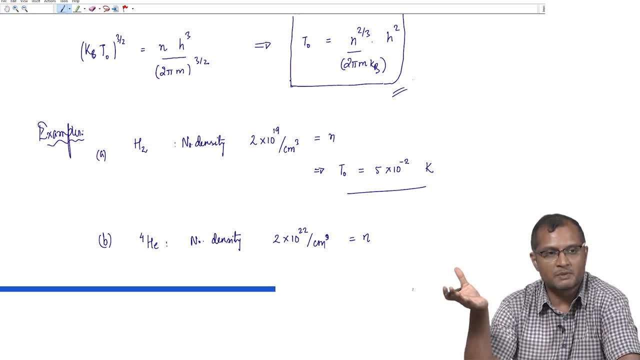 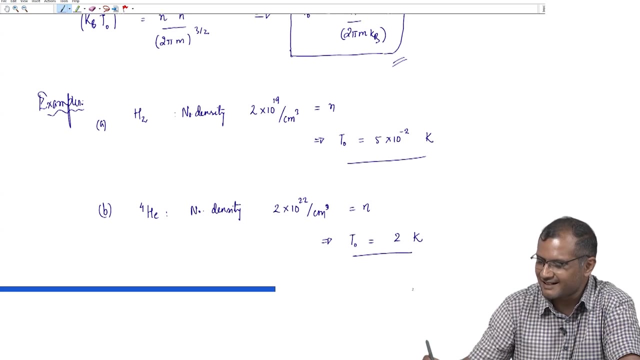 we have, you know, computed. put the value of Boltzmann constant and Planck's constant, You will find that the degeneracy temperature for liquid helium is of the order of 2 Kelvins, which is in some sense 100 times higher than the previous guy. previous guy was of the 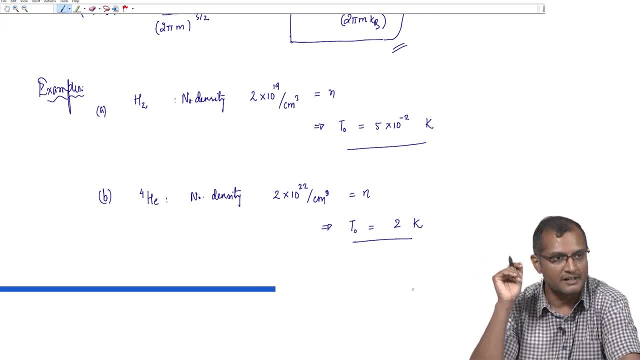 order 0.01.. This guy is of the order 1.. So already by boosting density I have actually made quantum mechanical effects come sooner, So I do not have to go all the way to 0.01 Kelvin now. 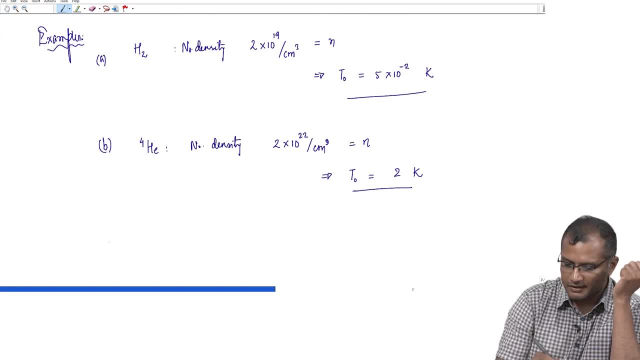 Ok, Going by this logic, you can expect trouble to come if you go to electrons in a metal. Now why these heat capacity expressions given by Dulong and Pettit do not work for metals, even at room temperature. It is because of this. 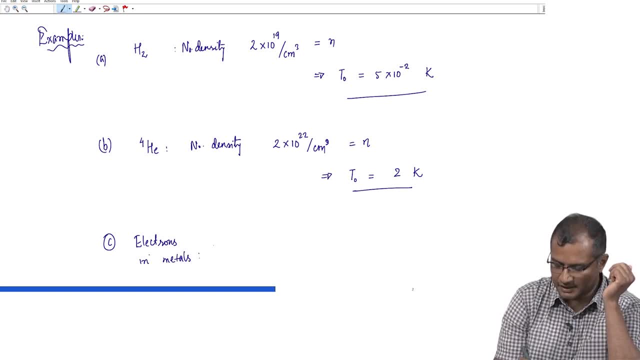 Ok, Let us do this calculation also. Now you take typical copper, for example, copper which is a perfect, you know perfectly good- example of a metal, and each copper donates one valence electron to the matrix. So a number density of a typical copper block is of the order of 10 to the power, 22 per. 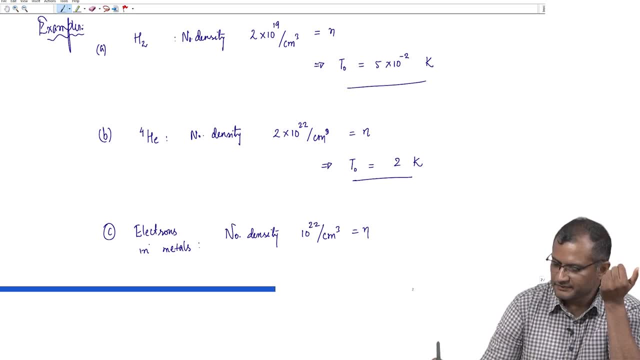 centimeter cube, Which is my density, That is, per meter cube. Ok, So if you take this number, density, and do this calculation, you will get well, as expected, because now I will get a degeneracy temperature much higher. This degeneracy temperature comes out to be 10 to the power 4 Kelvin. 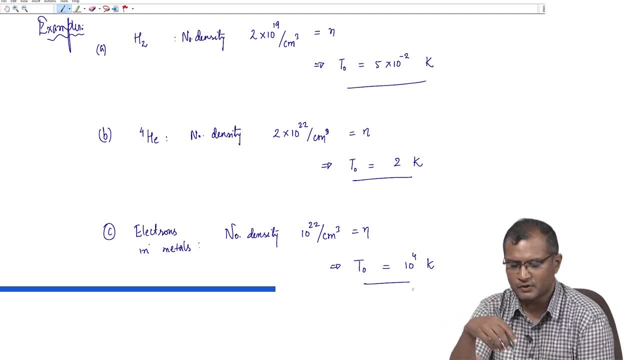 The reason why the two degeneracy temperatures for liquid helium and electrons in the metals I will explain later, Ok, Ok, So these two are so different, The electrons in the metals having such higher degeneracy temperature, in spite of the fact. 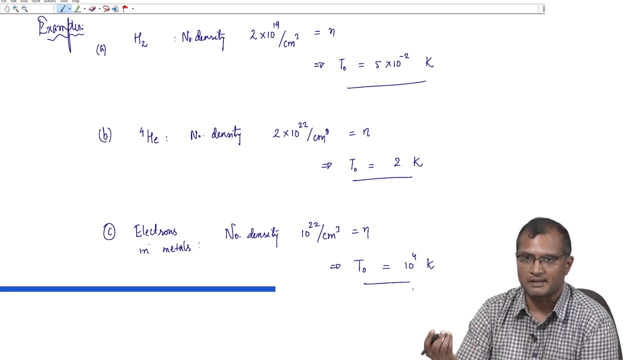 that both had the same number. density is because helium 4 has a much higher mass- ok, roughly 8000 times heavier than electron, because it has 4 nucleons, And so that is the reason why you have such different degeneracy temperatures. but the 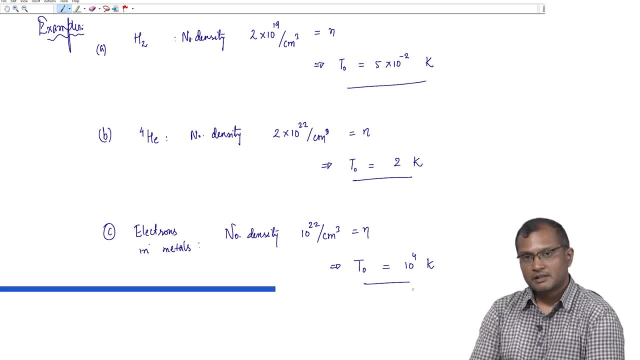 thing to see here is that for electrons in the metal, The degeneracy temperature, that is, the temperature where quantum effects will arise, is 10 to the power 4 Kelvin. This tells us that at room temperature, which is much below 10 to the power 4 Kelvin, we 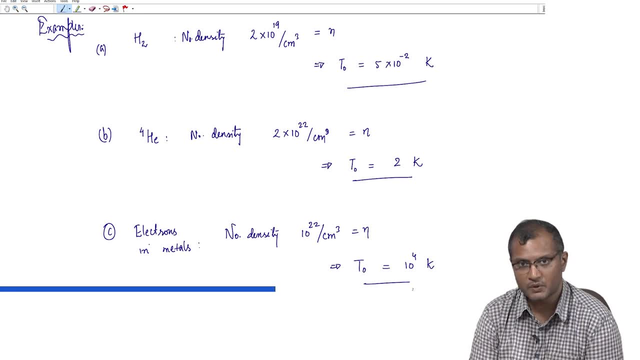 must invoke quantum mechanical theory to correctly understand heat capacity of solids due to these free electrons. Ok, Ok, Ok, Ok Ok. So the number of electrons in the metals has to be quantum mechanical. These electrons are heavily quantum mechanical at room temperature in the solid metals. 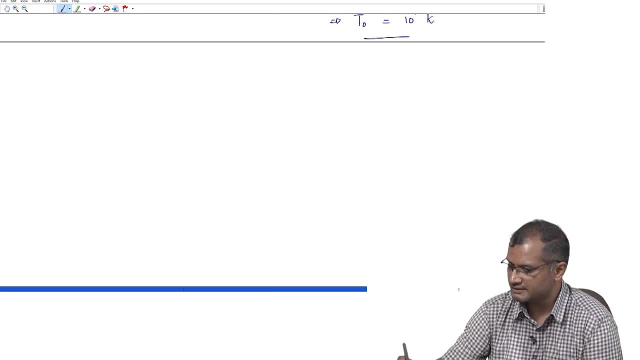 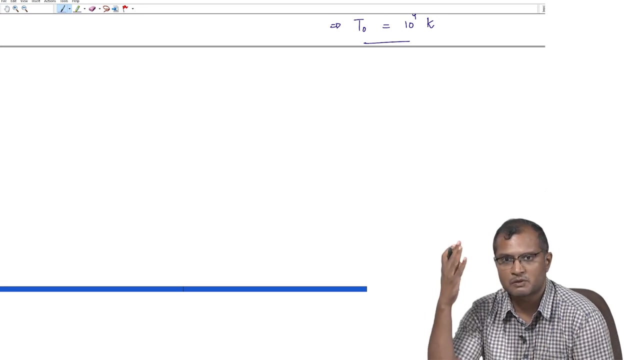 Ok, So that is the you know, that is. this basically gives you an a feeling of the numbers that I must invoke quantum mechanics when I am dealing with electrons and metals, because that is a degeneracy temperature. 300 Kelvin is for sure much, much lower than 10 to the power, 4 Kelvin. 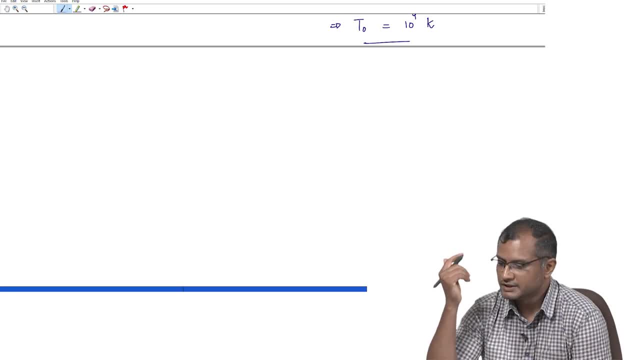 Ok, Ok, So only when temperatures are much higher than 10 to the power 4, you can include. you can use a classical theory of electrons in metals, but then at those temperatures you do not have a metal, You will probably be, you know, making a gas out of a metal. 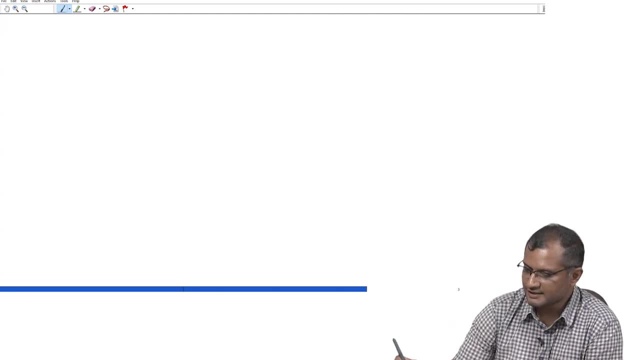 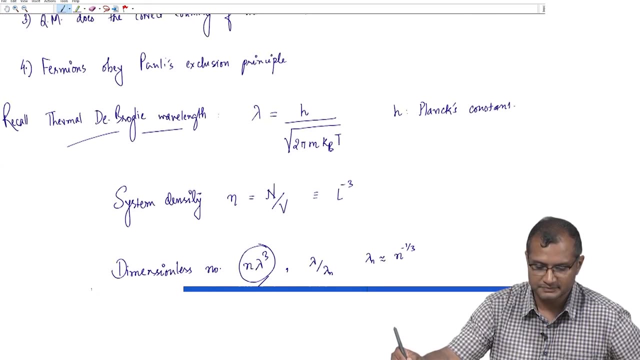 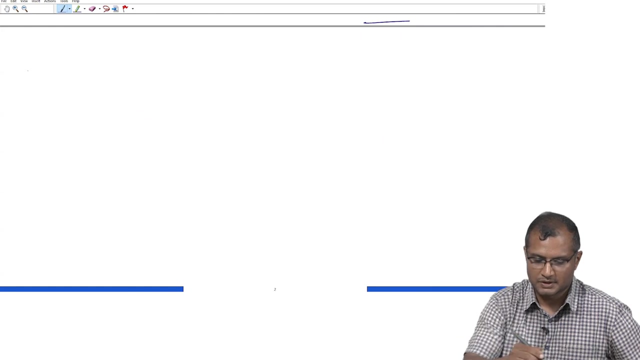 Right, So now let us proceed with the second topic in the agenda, which is: if you go back, So let us look at the statistics of indistinguishable particles. Ok, So indistinguishable particles are handled very carefully in quantum mechanics. 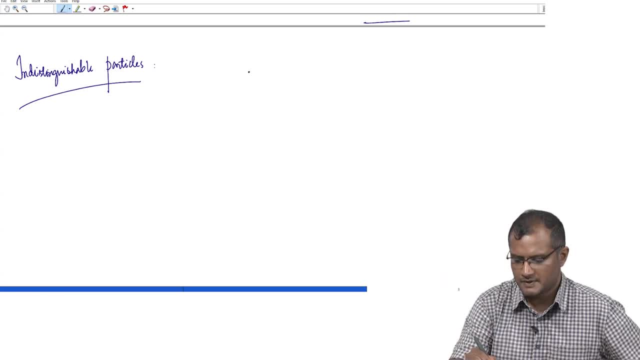 For example, if I take just the two particle system, So one is somewhere, location R 1, and another sitting at location R 2, just take the two particle system. Ok, So I am just taking a two particle system, Then I can write down the wave function of my system as the two of the two particle system. 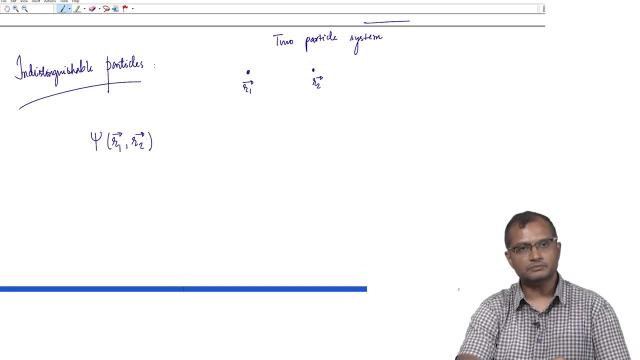 as psi of R 1, R 2.. And This is the system wave function. I will show how to write down psi, which is the overall wave function in terms of single particle wave function. in short while. but I know for sure that if I permute these two particles, that if I make you know R 2, second particle, 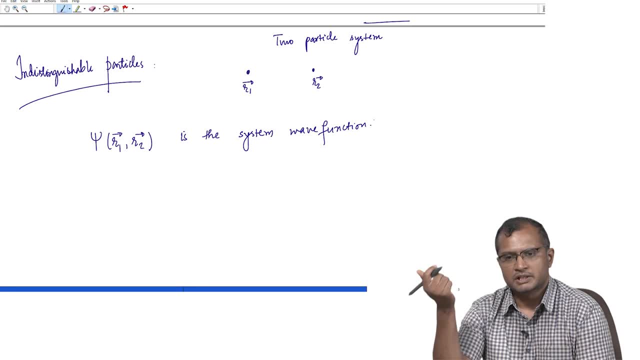 go and sit on R 1 and the first particle go and sit at R 2. So it will fail. Ok, So the Hamiltonian of the system does not change. ok, because the Hamiltonian of the system is a function of potential energy and kinetic energy and clearly, if the particles 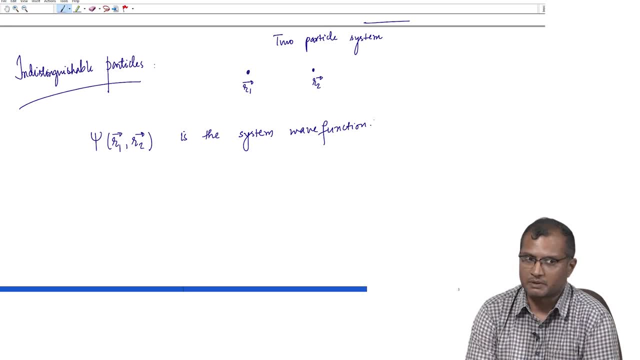 are indistinguishable. I am not affecting their potential energy in any way because they are the same particles. So permutation of 1 and 2 has not change the potential energy and it clearly does not change the kinetic energy. ok, because I am just putting one particle having some kinetic 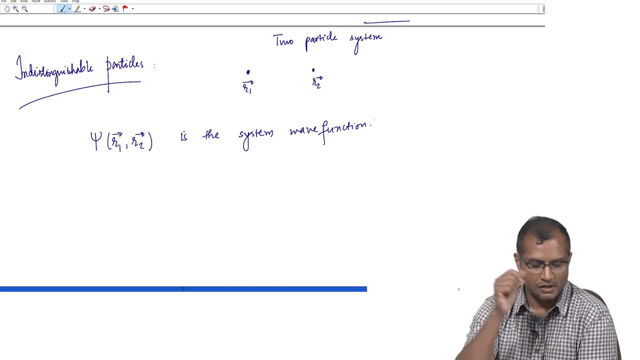 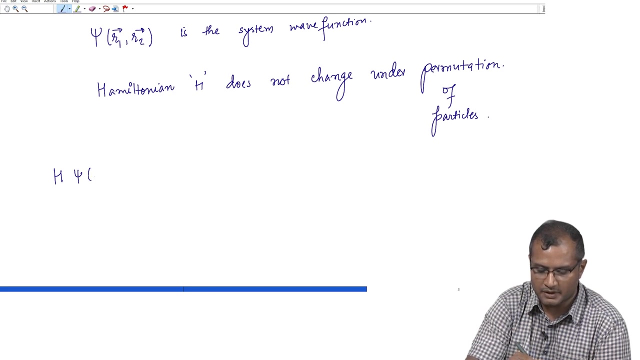 energy at location, which is different, Kinetic energy remains the same. Ok, So Hamiltonian does not change under permutation of particles. ok, Meaning what? The energy of the system remains the same under permutation of particles. This essentially means that if I take the Hamiltonian operator and this 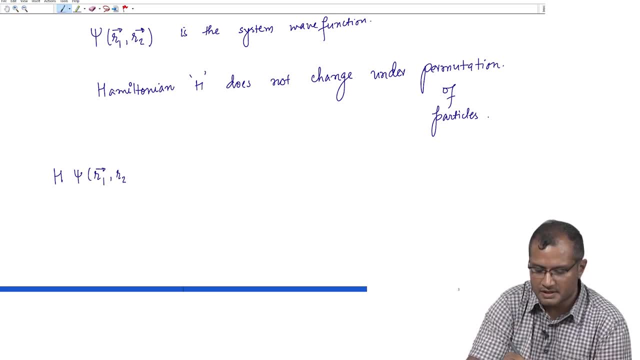 and operates on the particle to particle wave function. the eigenvalue by the total energy of the system does not change if the particles are permuted. Ok, That is the meaning of the Hamiltonian operator, which means: if I, if I think of a. 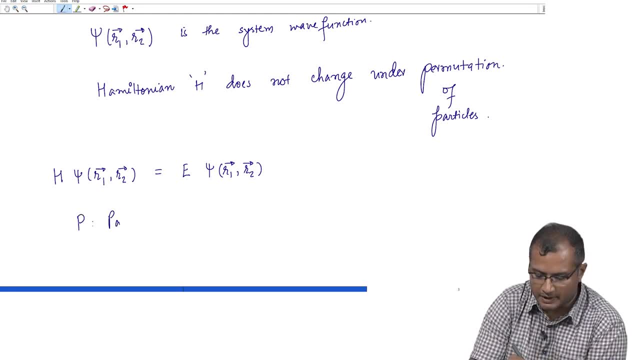 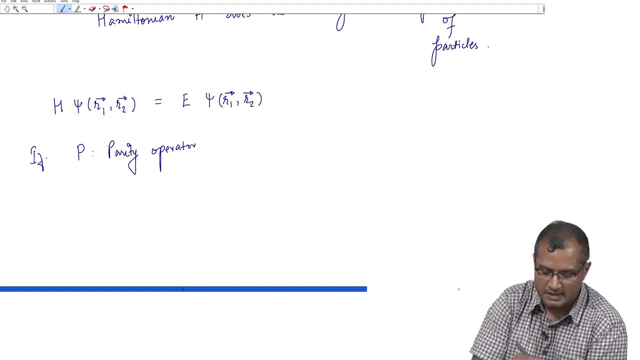 parity operator, P being the parity operator whose action is to just permute the particles. ok, Then I do not expect to see any change in energy, which means the parity operator, when it adds on the system, makes the wave function basically psi of r 2, r 1, simply swaps. 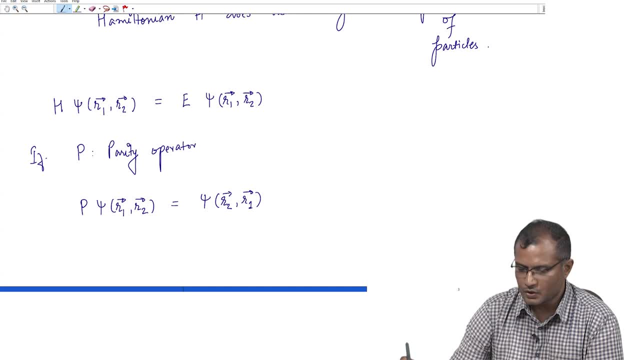 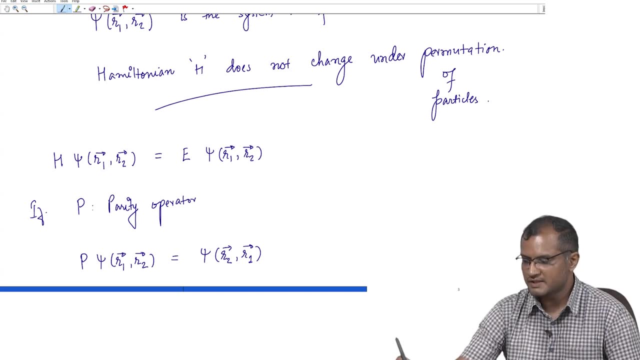 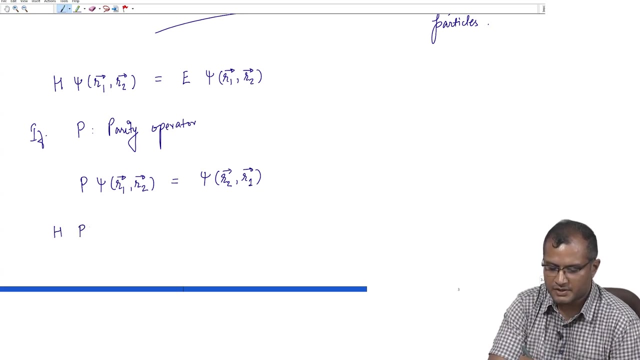 the two particles at the effect of the parity operator. And I know from what I have written here that the Hamiltonian of the system must not change, which means the energy of the system should not change. So apply the Hamiltonian operator on this new wave function P of psi, ok r, 1, r, 2, considering 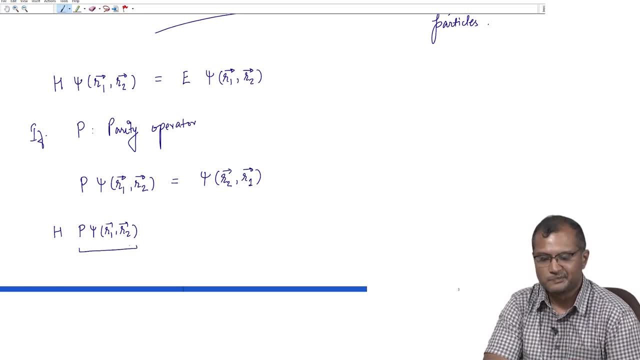 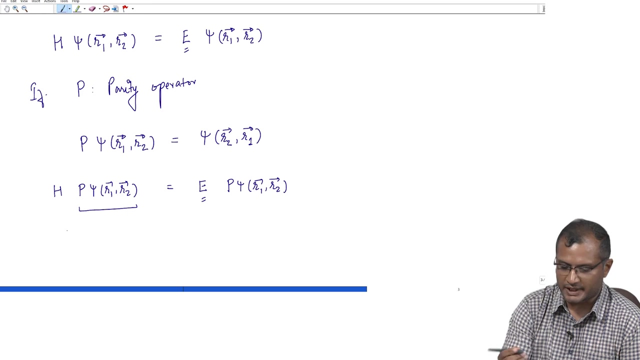 this as my new wave function. ok, Then I must get the same energy, because the energy has not changed. ok, So the same function. wave function comes back, without any change in the energy. This E is the same as this E. ok, But I can also write this. as you know, I can also consider P operating on h psi, ok, So 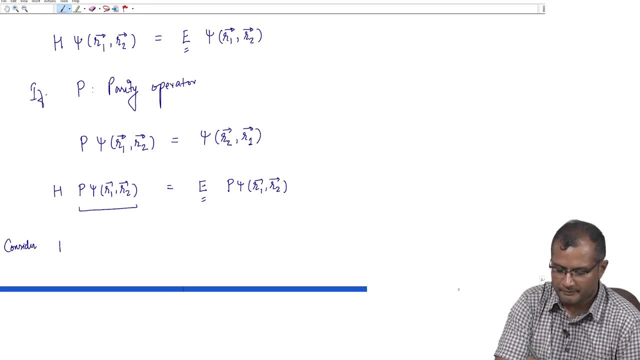 this is my new function. this is nothing but P h on psi is simply gives me E times. in that sense, That is the. so this is the first one piece hole right. 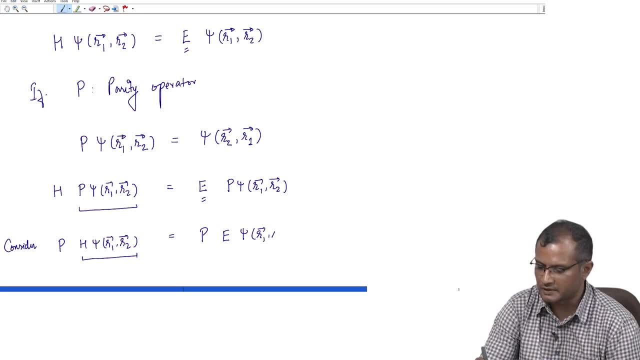 in. that is the eigenvalue: psi r 1, r 2, but E is just a number, it is the eigenvalue, So I can write this as E times P operating on psi r 1, r 2, which is nothing but psi r 2. 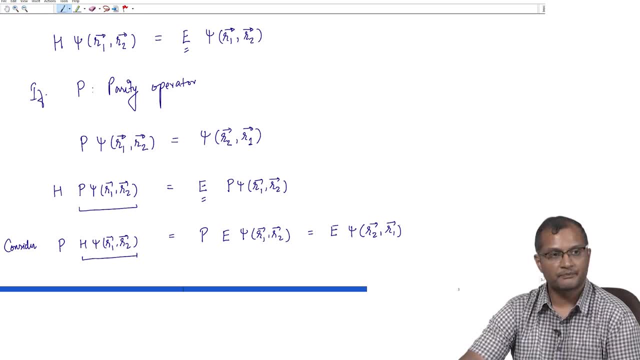 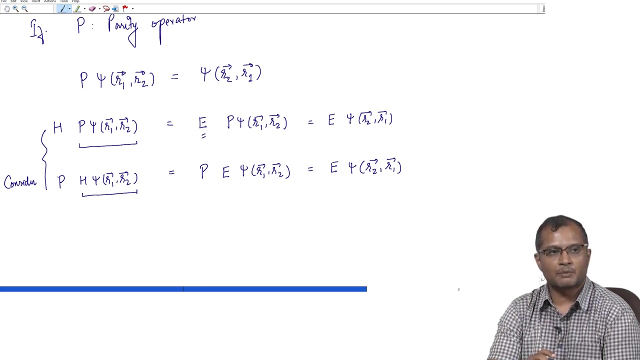 r 1. ok, You can compare the previous equation. this is also E of multiplied to psi, of r 2 r 1.. So if these two are same, I can say that by looking at these two- the left hand sides that my Hamiltonian operator commutes with the 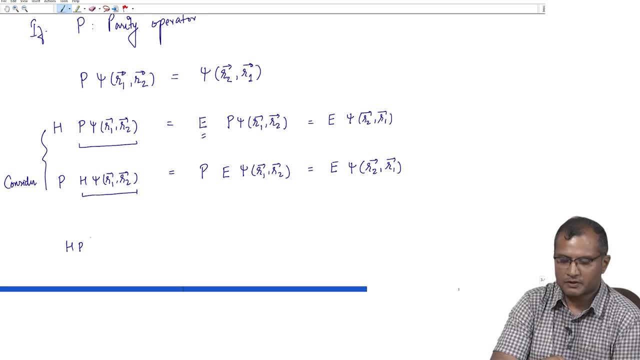 parity operator, I can say that the product of these two operators is the same as product of P and H, Implying that the Hamiltonian operator commutes with the parity operator for our identical particle system or indistinguishable particles, and this has a very important consequences. This is why quantum mechanics does calculations. 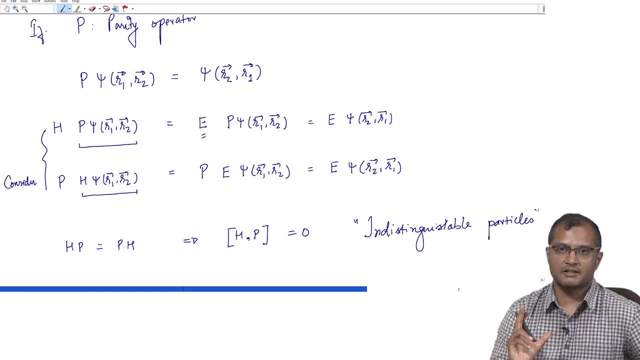 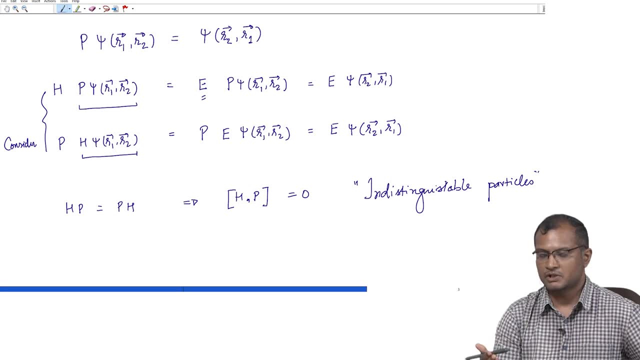 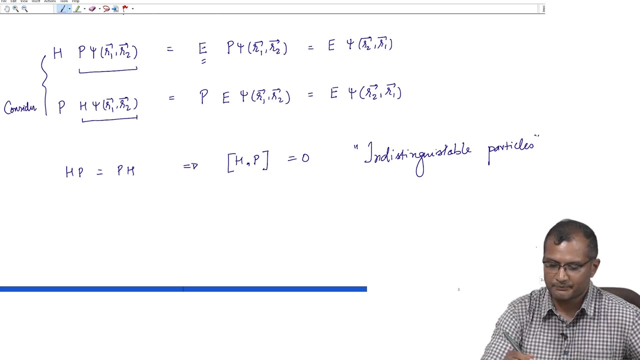 correctly. ok, This is the birth of the correct enumeration of states In a very logical way, very logical sequence of steps. I showed that the Hamiltonian of the system commutes with the parity operator. This brings us to the stage that I can write down now the effect. 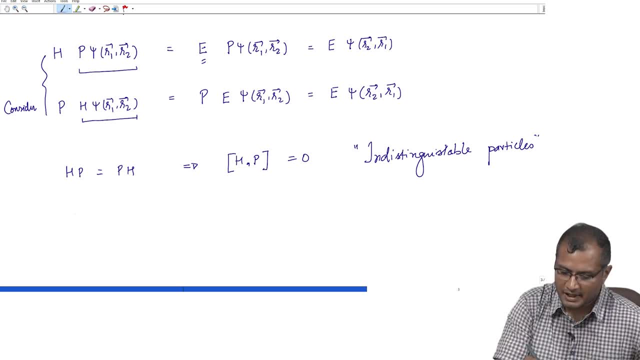 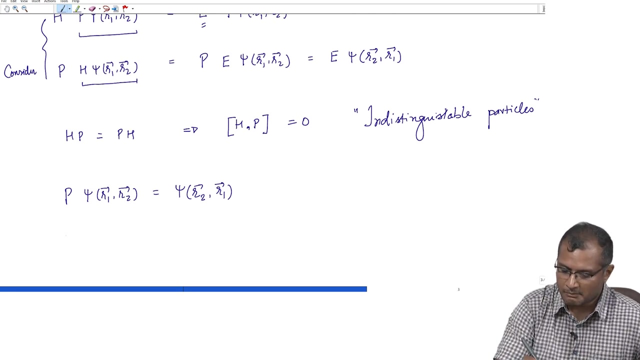 of my parity operation done twice. I already know that P simply swaps the positions. So P operating on psi r 1, r 2 simply gives me the same wave function now, but the particles are inter permuted. If I do not know what is this new psi, I can compute this new psi. 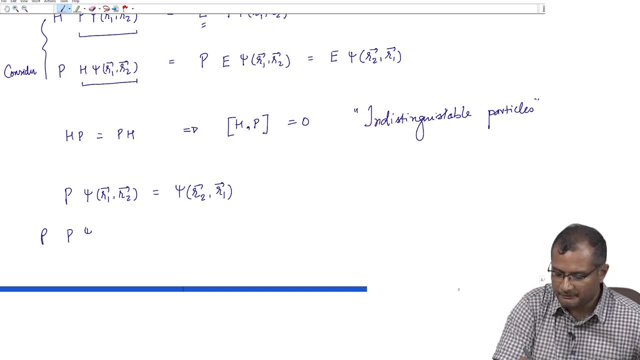 by operating in P again which is nothing, but P square operating on psi r 1 r 2, but I already know what is P operating on psi. Your side is opposite again, you are that side. That is when youways have arechted solution to the post- �, where P is egal to you, meaning 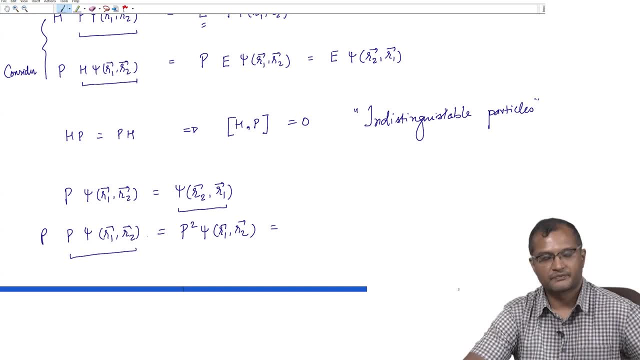 W too is in your side. so this is säga fathers also ours. So now you are at the relationship you are happy with. condemment to Sh τον Ken, music again, which was nothing but p squared operating R 2, R 1.. So one more operation of P on this will give me back the old function. it will. 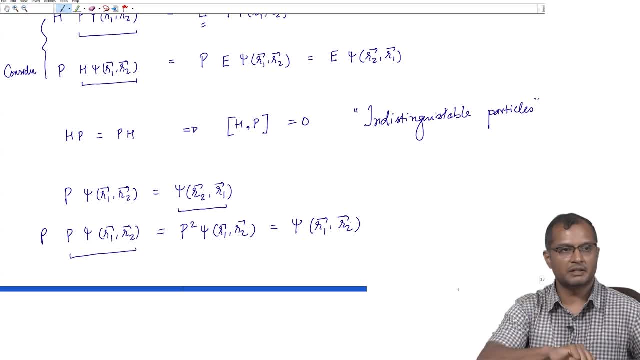 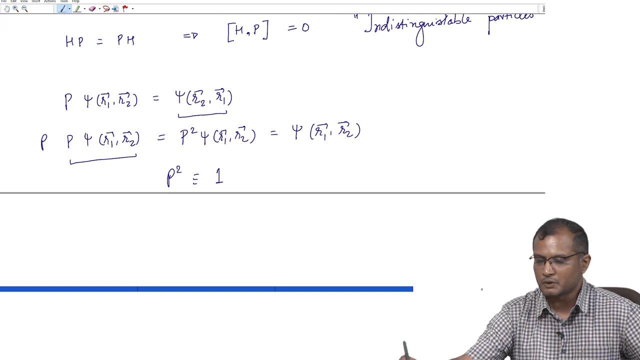 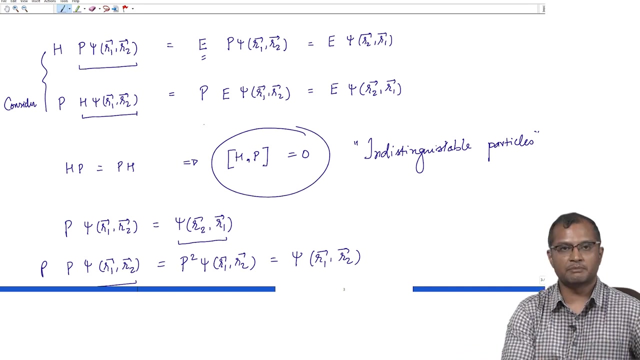 bring the system back to the old state. You made 2 go and sit in 1, you do one more permutation, you get back the same old wave function. So definitely my P square as an eigenvalue, which is 1, and the fact that permutation- you know, you have seen that here, that the Hamiltonian 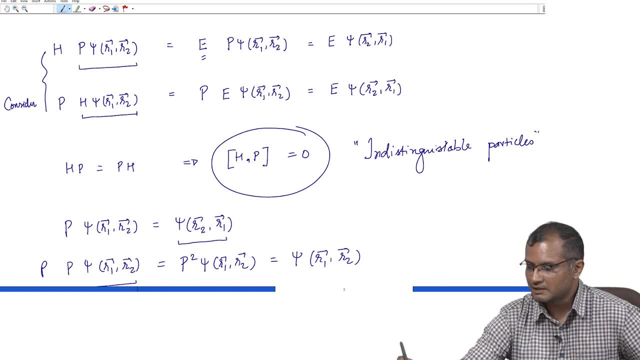 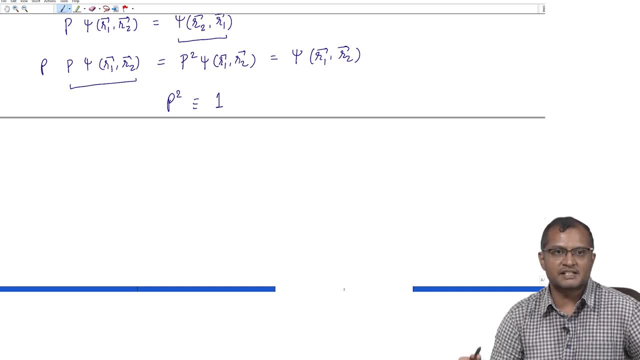 permutes with the parity operator tells me that a permuted wave function has a same energy and hence it is the same state as the previous state. if there is no degeneracies, ok, Then there are. this is the same state because it has the same energy, same. 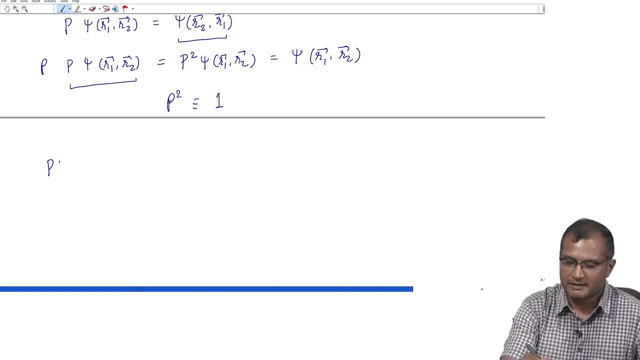 So this is the state of the same state, because it has the same energy, same Hamiltonian, which means P, psi and psi differ only by some constant pre factor. ok, It is. 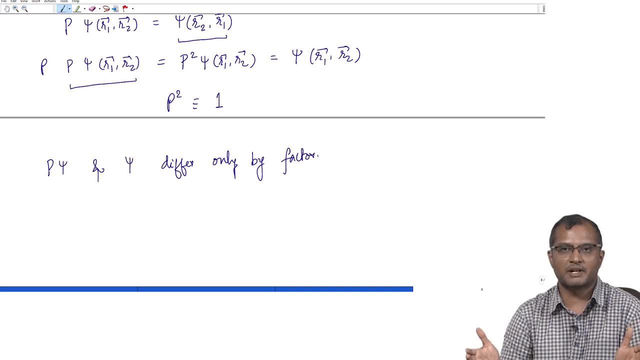 just the same, because if I take P, psi and psi, they should be differing only by a constant pre factor. So the eigenvalue equation is not moved. you have the same pre factor on both sides. H operating on P psi will giving me some E operated on P psi. They are the 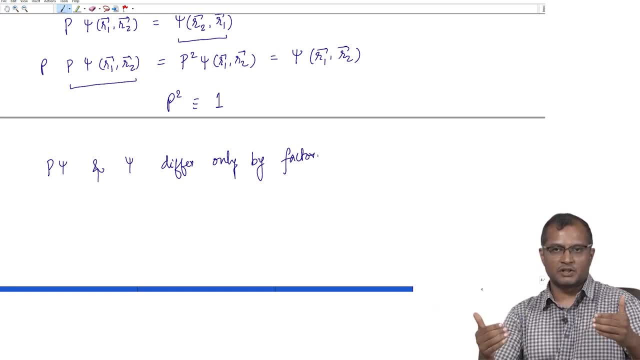 same. you know, if P psi differs from psi by just a factor, you are looking at nothing. but H psi equals to E psi. ok, You can knock off that constant pre factor both sides, which tells me that my operator P should have the eigenvalues plus or minus 1.. That is the only. 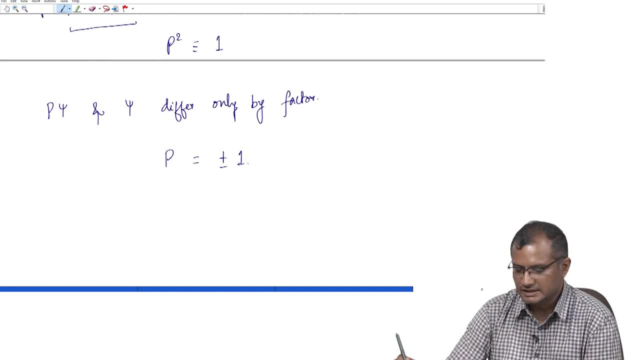 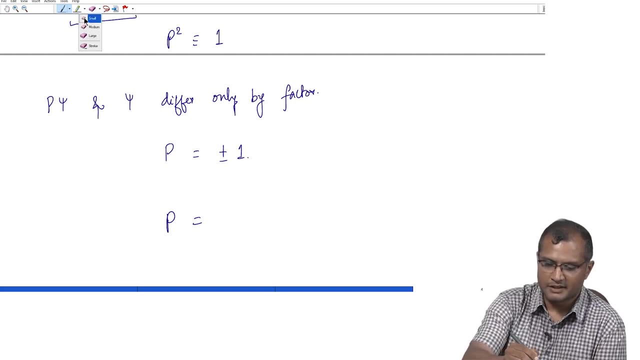 way I can make P square 1,. ok Now this basically leads to two definitions. So, if you have, you can define particles or system of particles which have the property of the action of parity operator on the whole system, giving an overall positive sign, which means not affecting the system as a system. 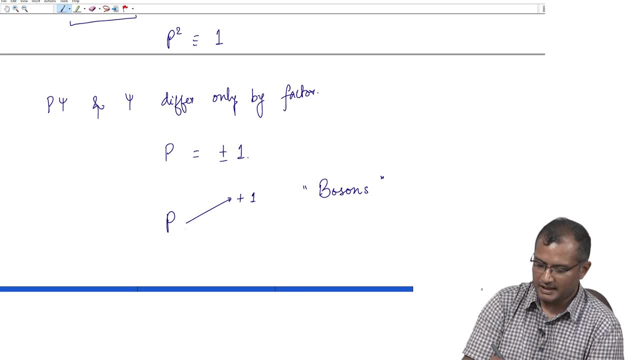 of bosons And define the other type of. there is only two possibility, plus and minus 1 as a system of fermions, And this is only a definition. by the way, you can swap the definition. you can call P plus 1 as fermions and P minus 1 as bosons, And everywhere your fermions. 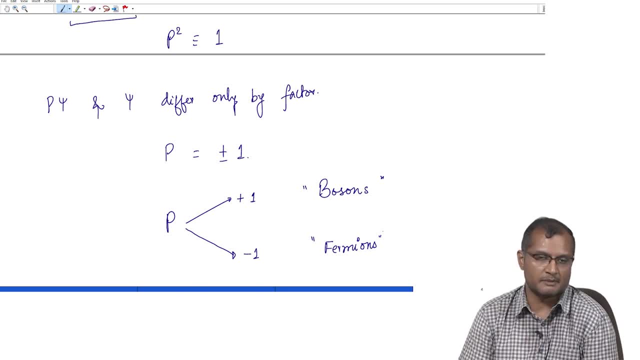 will obey the Bose statistics and bosons will obey the Fermi statistics. So this is what is in a name, What is basically to be realized at. Ok, These types of particles in the due course will be shown to obey a statistics of average. 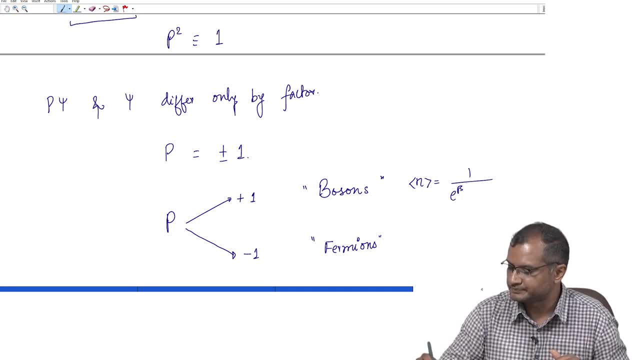 number density going as 1 upon e to the power beta, some jth level: E j minus mu minus 1.. And these guys will be shown to have statistics which is 1 upon e raise to beta: E j minus mu plus 1.. ok, 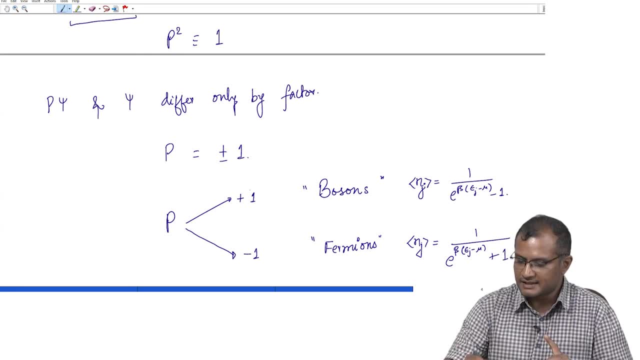 So what is essentially is that this should match with this and this should match with this. you can call bosons and fermions either way, I do not care, but the guys that commute with the parity operator, the wave function of the guys which commute with the parity. 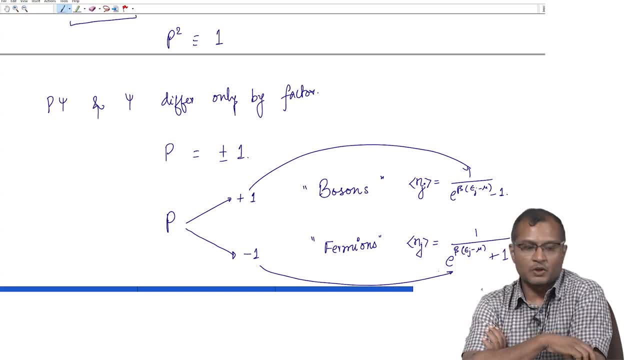 operator and for which the parity operator has an eigenvalue plus 1, I will call them as bosons for historical reasons, and they will be shown to have statistics which go like this and the other guys will have statistics written below. you can call whichever what. 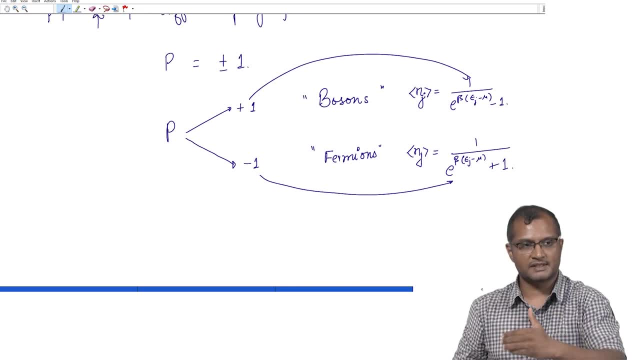 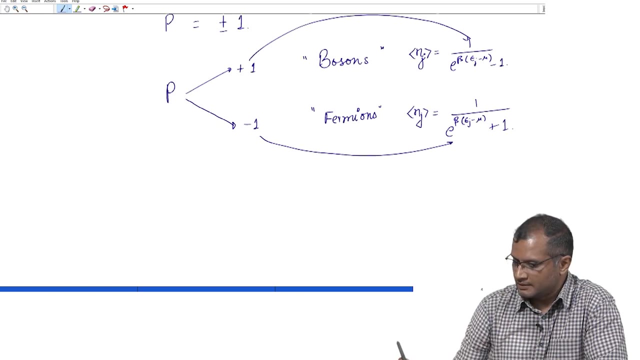 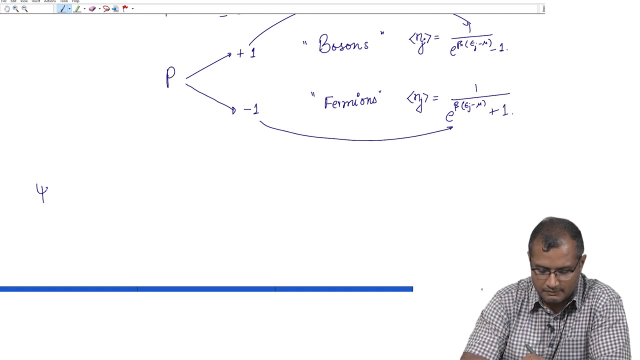 you want, but historically we call them the first class as bosons and the second class as fermions. So it is important that this map is between the values of the parity operator and the current statistics. Now we can write down the wave function of the system, this two particle system, as some 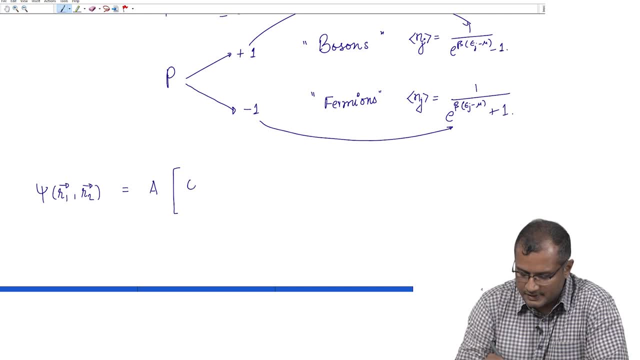 kind of a linear combination of single particle state. So I will take. what do I mean by single particle states is the following: So let me first write down, So let me first write down the single particle, so draw a figure, so to write a psi. we consider: 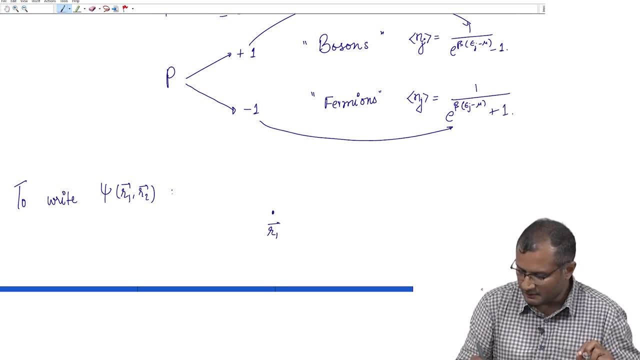 two single particle states. So I have one particle at location r 1 and another particle at location r 2. meaning of single particle state is that I can consider two localized wave functions At the location of r 1 and r 2.. 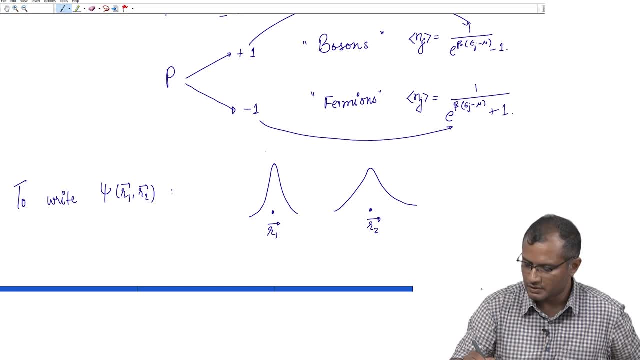 So maybe you have another wave function which is localized at r 2. call the first one as phi 1, call the second one as phi 2.. Classically you have a particle there at r 1 and r 2. quantum mechanically it is represented. 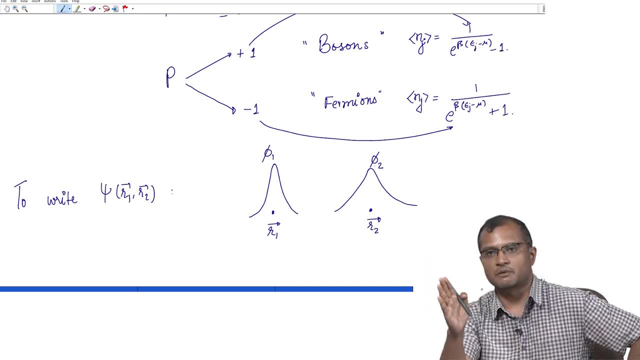 by a wave function which is localized around r 1 and r 2. ok, So it is non deterministic quantum mechanics. So I must, So I must. So I have n particles in this room. I have n single particle wave functions, each one. 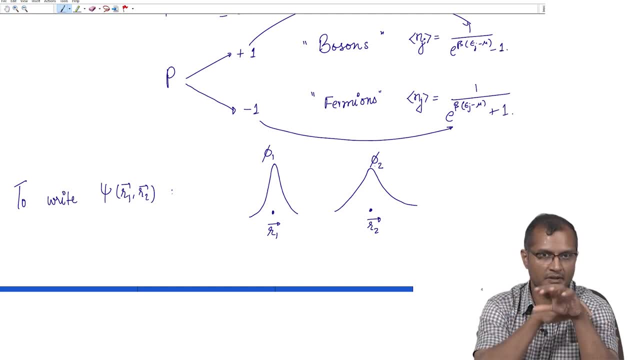 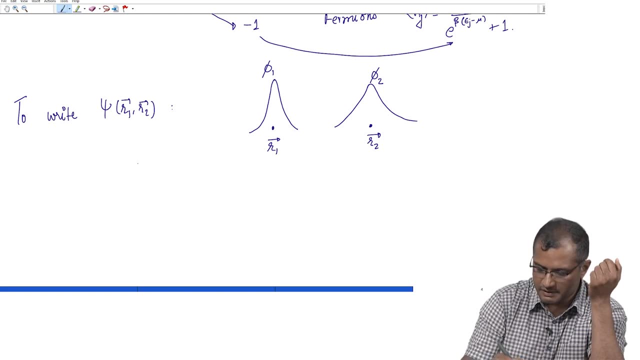 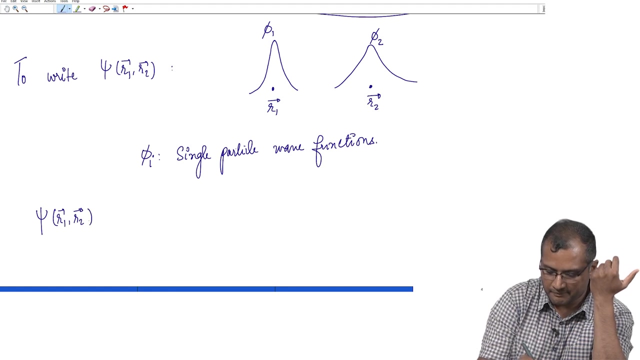 of them localized around the particle, physical location of that particle. So you can write down psi in terms of this phi. So these phi i's are basically the single particle wave functions As simply some normalization constant into, you know, the only linear combinations that. 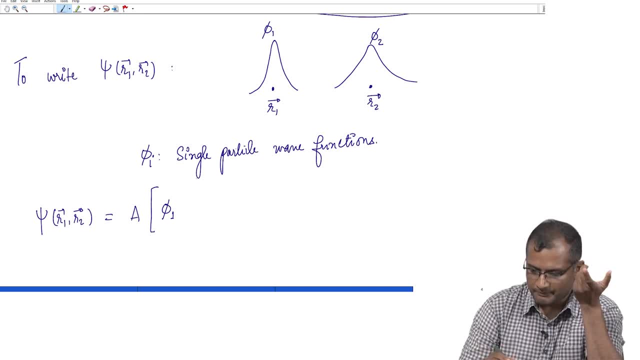 you can construct, basically are products of phi 1 and phi 2.. So I will take phi 1, r 1, which is like the first particle, Which is like the first particle sitting at location r 1, into phi 2, because this is the 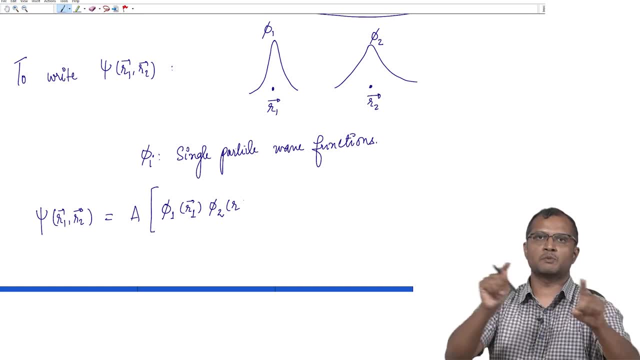 joint probability. So the fact that my system has two particles at r 1 and r 2 is the given by the joint product of phi localized at r 1 and phi 2 localized at r 2. ok, is that it for two particles I have? 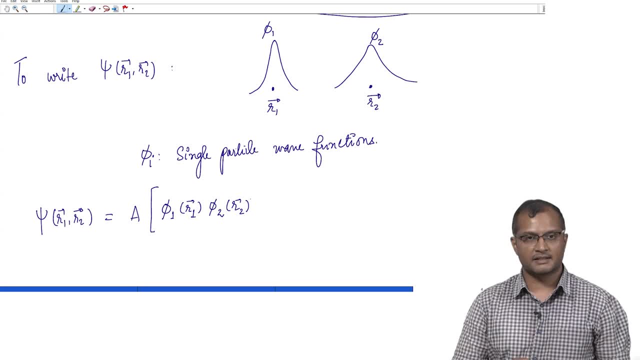 one more possibility. Ok, So the second particle can sit at r 1 and the first particle can sit at r 2.. So that is given as phi 1, r 2 into phi 2, r 1.. See phi 1 and phi 2 are localized wave functions, one localized at r 1, the other localized at 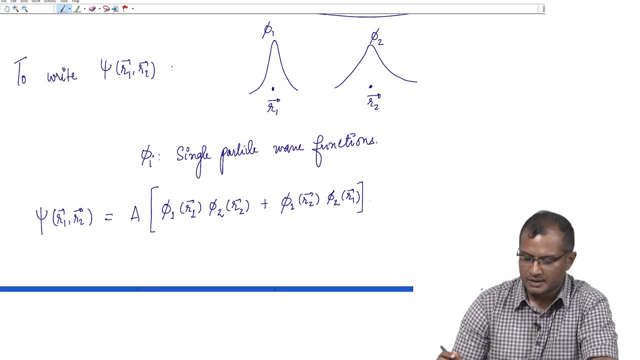 r 2. We have simply swapped the particles. ok, This is for bosons. if I were to write down this wave function for fermions, I have to take a negative sign here. Why? Because if I take a positive sign then that would mean that under permutation of the particle, 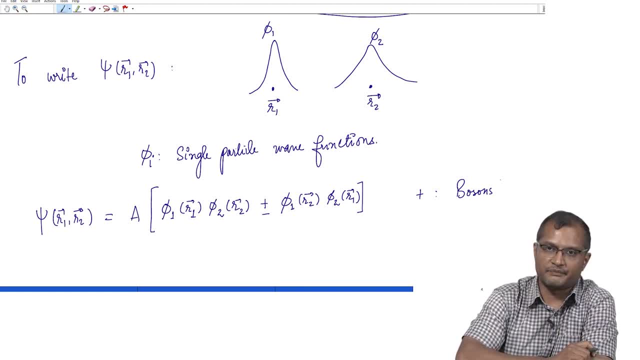 the wave function is not incurring any overall negative sign, which means plus sign has to be for the bosons. Ok And Ok. So these two particles are fermions, they are under permutation. of the two particles the overall wave function should incur a negative sign and that is only possible if I write down. 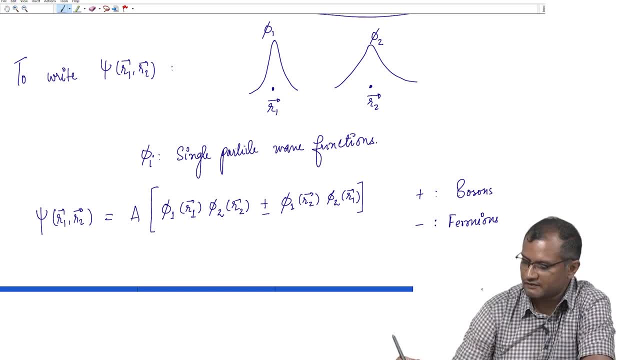 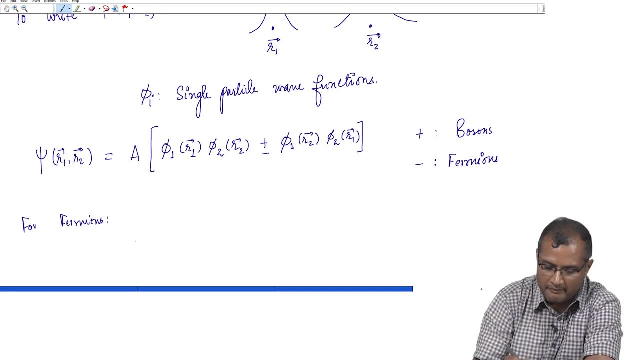 the second product with a negative sign. So now you can see, for fermions, if I swap r 2 with r 1.. So for fermions, so if I apply the parity operator on r 1, r 2, this will give me a times. 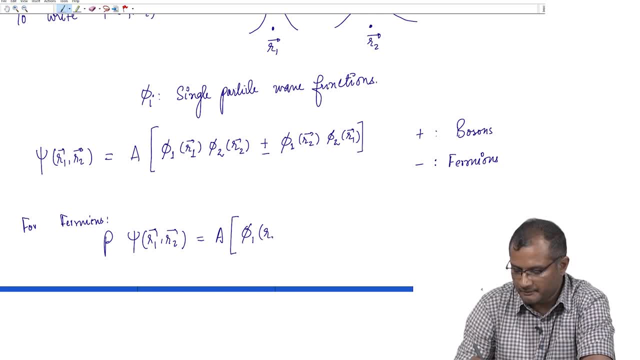 phi 1 r 2, phi 2 r 1, and I have to take the minus sign minus phi 1 r 1 into phi 2 r 2, but this is nothing but minus of r 1.. Ok, Ok. 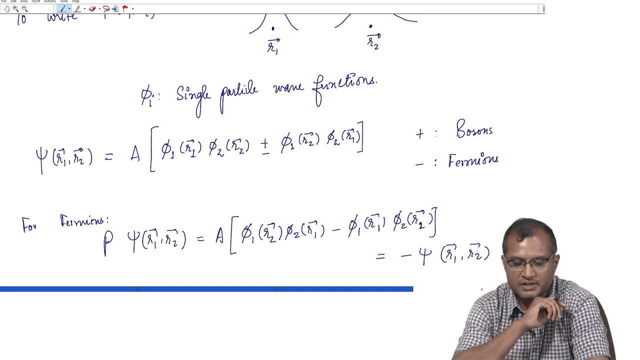 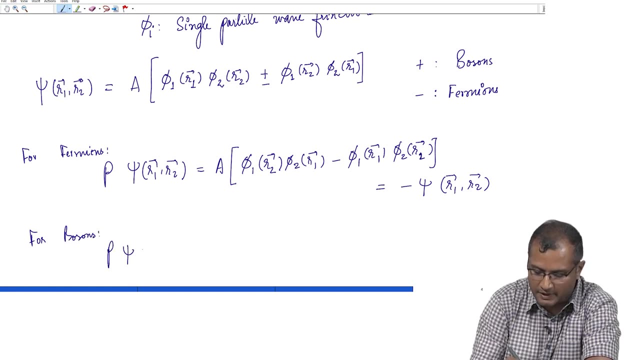 Ok, So this is my original fermionic wave function. Ok, So this is what I expect similarly for bosons. if I apply the parity operator, then I get back the same function: phi 1- r 2, phi 2, r 1 plus r 1- r 2.. 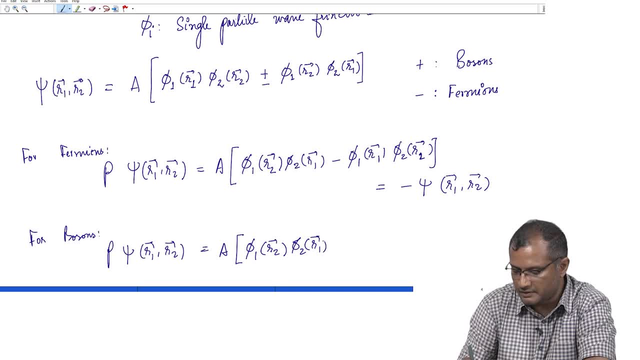 Ok, Ok, Ok, Ok. So that is why I have to take the plus, because I have a plus sign for bosons. Ok, Already given here. Ok, Hmm, Plus phi 1 r 1 into phi 2 r 2, but this is nothing but the old wave function. 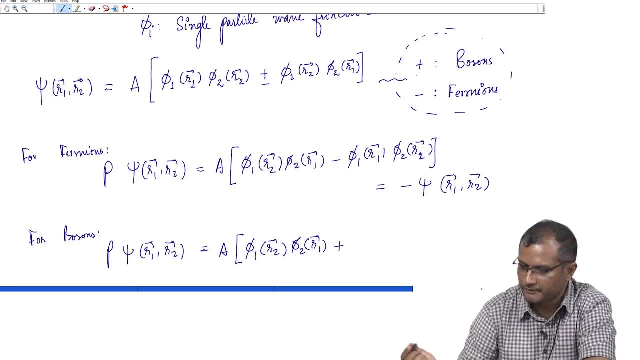 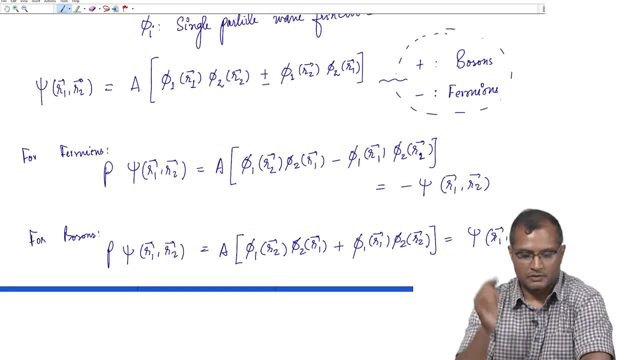 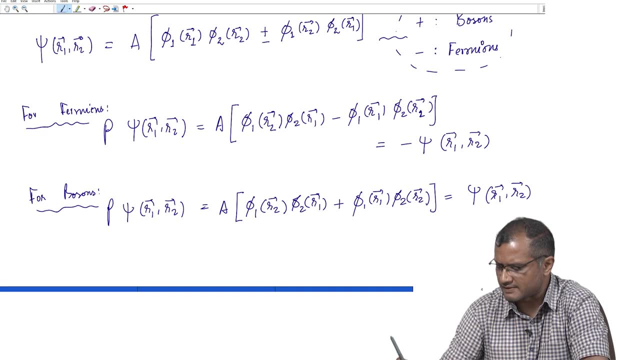 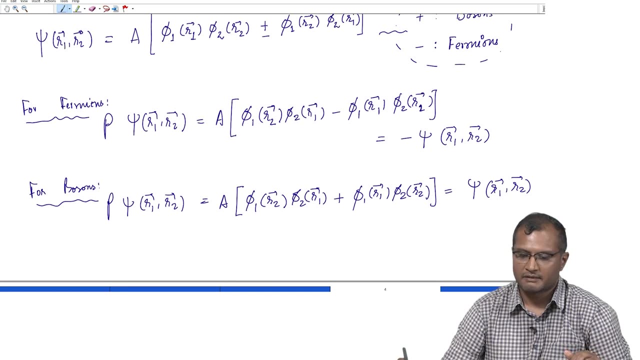 Ok, Ok, Ok, Ok, Ok. So this is why for fermions I have to take a negative sign. now it you can generalize this for 3 particle system, 4 particle system, n-particle system. So you can always write down the n-particle wave function by choosing 1 product and simply. 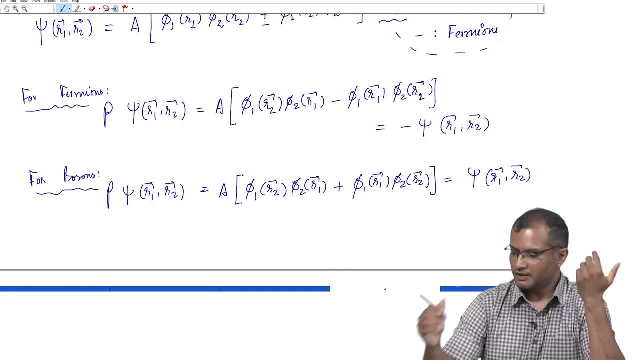 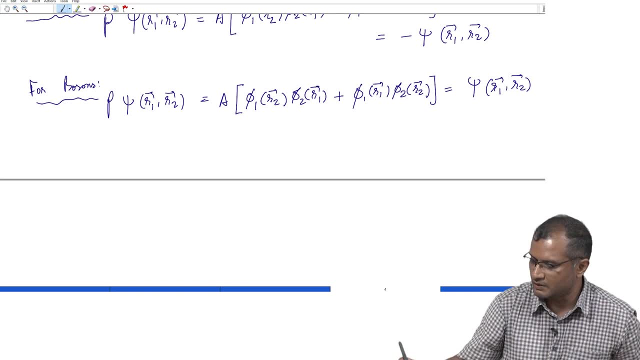 doing permutations of these products, and this way you can write down 8 in the determinant form, which is called as the slator determinant form for the 2 particles. I can thus write down what I have written for the fermions, only for bosons you do not, you cannot write using the determinant form. 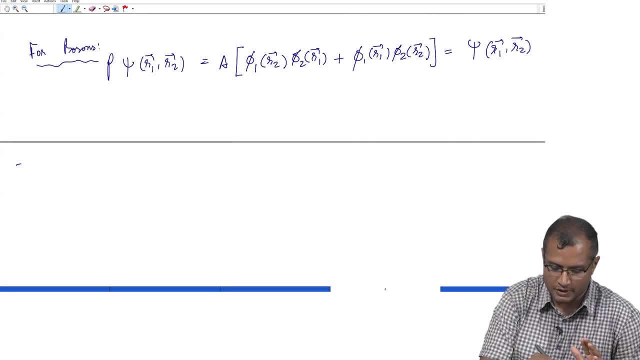 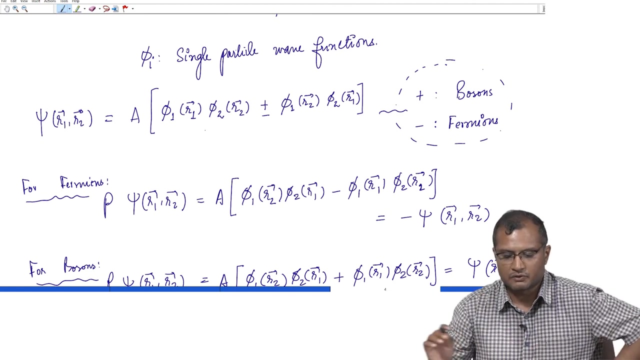 for bosons you just have to use a plus sign throughout. So for 2 fermions that we have just discussed, you can write down these, this wave function also in the determinant form. what I have written here, this particular, this equation: a times phi 1- R 1 into phi 2- R 2. 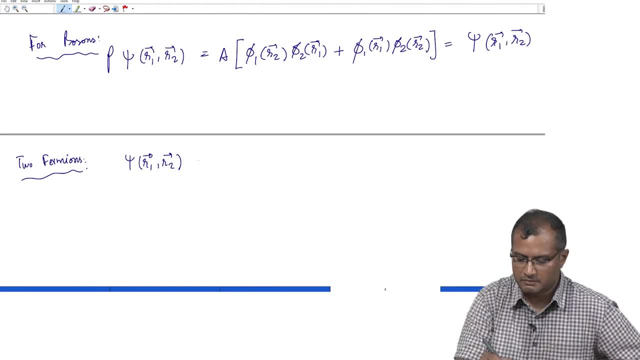 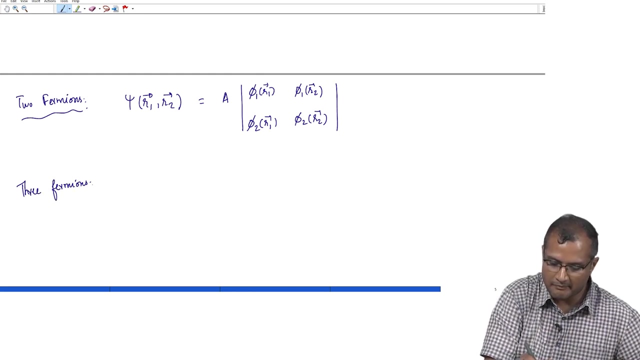 minus phi 1 R 2 into phi 2 R 1 in the determinant form. you can write it as a times a determinant phi 1 R 1.. So this is the determinant form And similarly for 3 fermions, or I would say for n fermions. let us write down for n fermions: 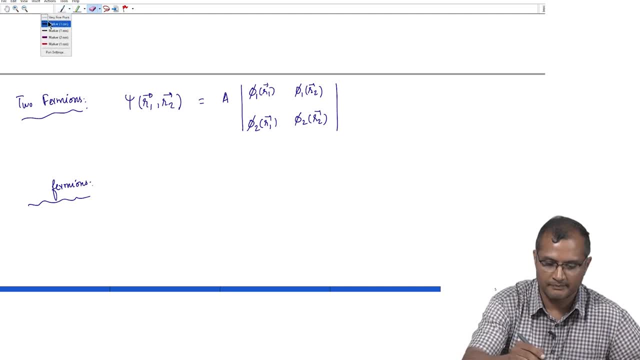 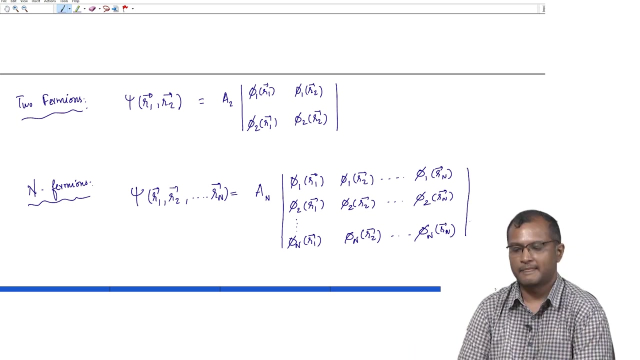 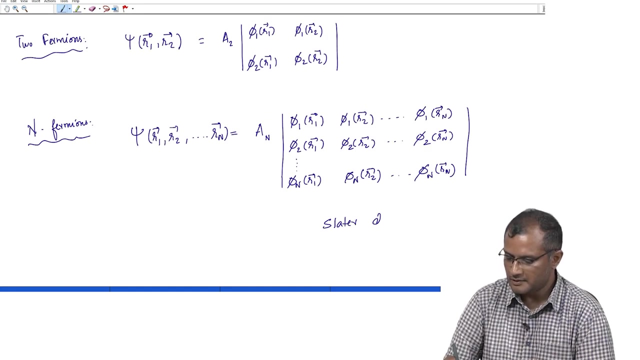 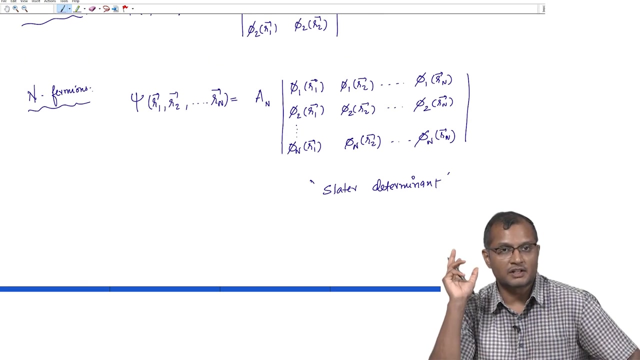 directly. you can write this n particle wave function. For historical reasons, couple of things to be, you know, sort of kept clear. here is: what is this normalization constant? ok, So we can work out the normalization constant by: and this will give us the n factorial you. 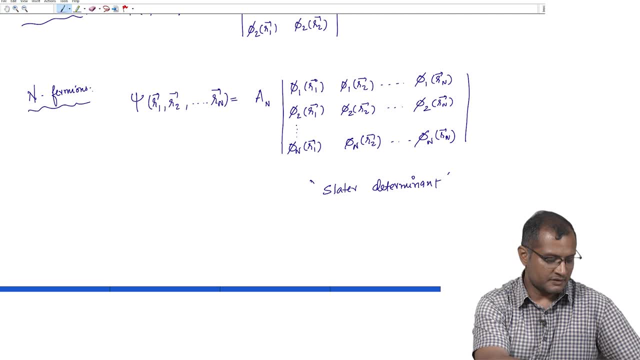 know logic. You see, for 2 particles, For 2 particles, how many combinations could you construct: 2, 1, 2 and 2: 1. with 3 particles you had 6, because that is 3 factorial. So with n particles I can construct n factorial. 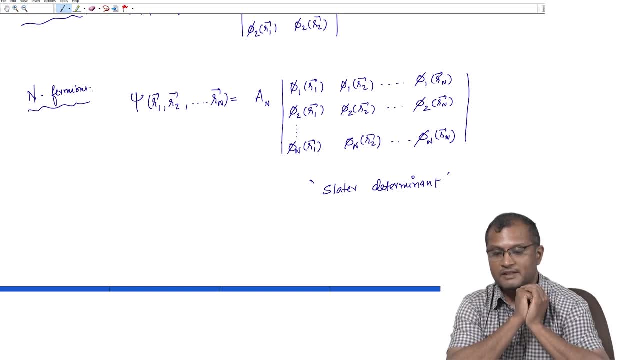 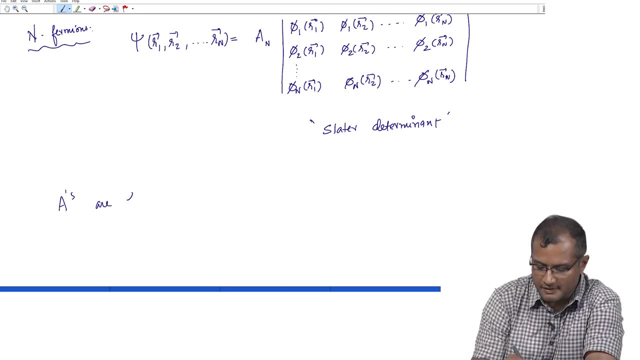 permutations. So this normalization constant is fixed. ok, So this a is are fixed by the normalization. So this is a very simple formula that you can write this down as a 1 over n integral, that your integration over the entire volume. ok, So I will take volume. i going from 1 to 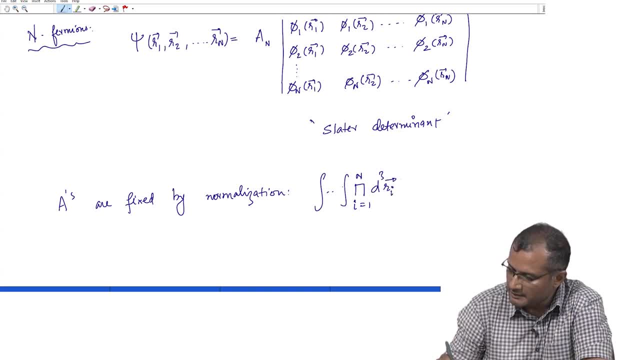 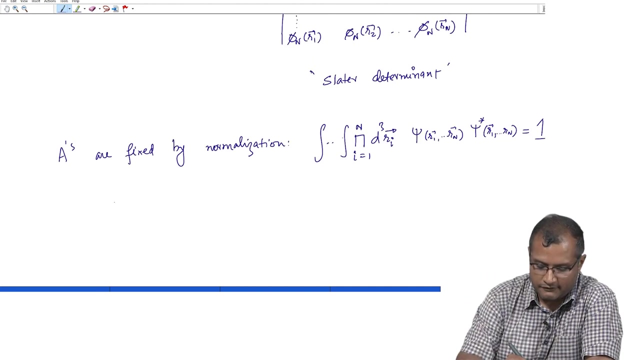 n d cube r i psi is now n particle wave function. ok, psi psi star is equal to 1, this is my normalization. So volume integral of psi psi star is 1,. ok, So for example, in 2D I can think of A 2 as just 1 upon factorial 2 to the power. 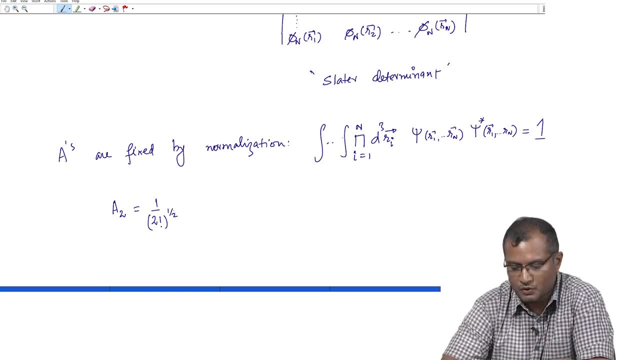 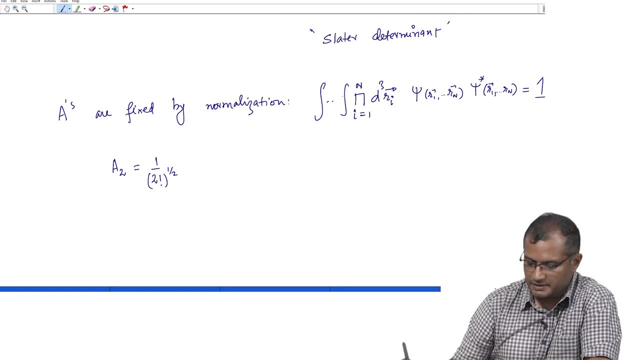 half, because when you do a psi psi star, this will become 1 upon factorial 2 and precisely. you know the. So the normalization on single particle wave functions also need to be specified here. I am going to write down with this: single particle normalization is given as: and that is very simple to see why you have you know. 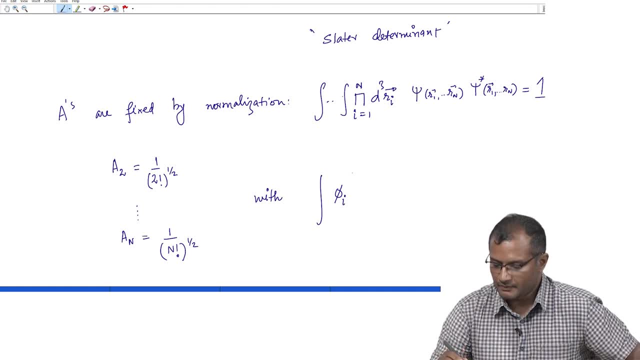 the sort of a orthogonality of the single particle wave functions. So this is the orthogonal scalar product. ok, So the orthogonality of the functions are basically represented as this integral phi with its complex conjugate, given as the 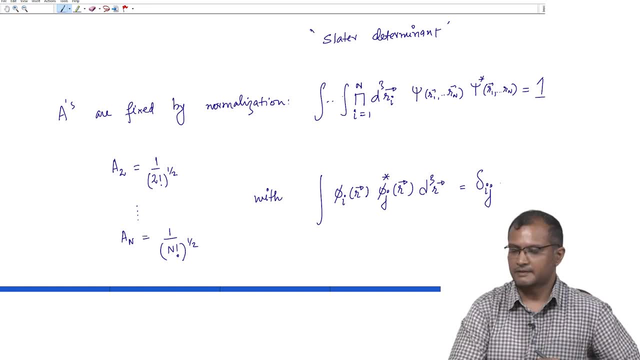 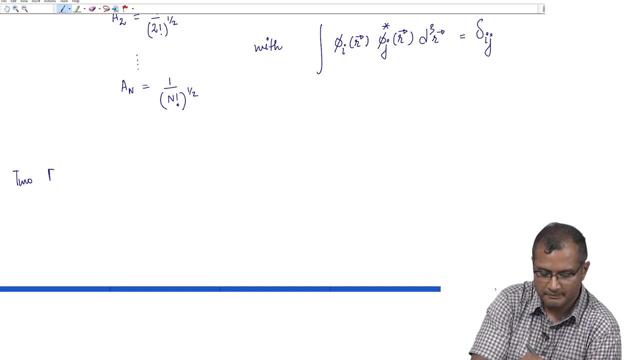 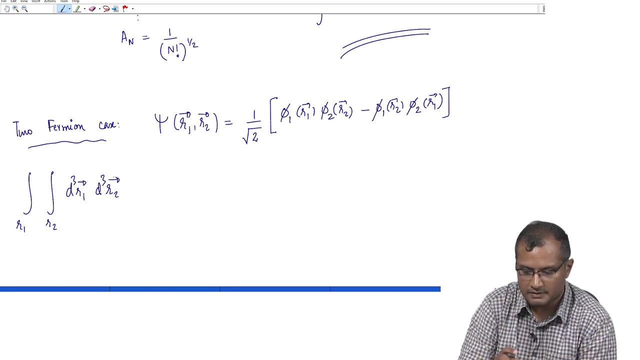 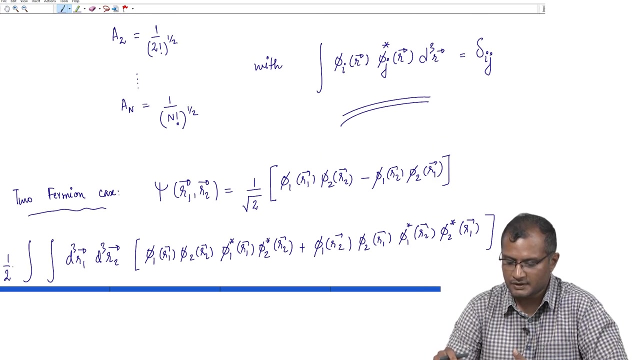 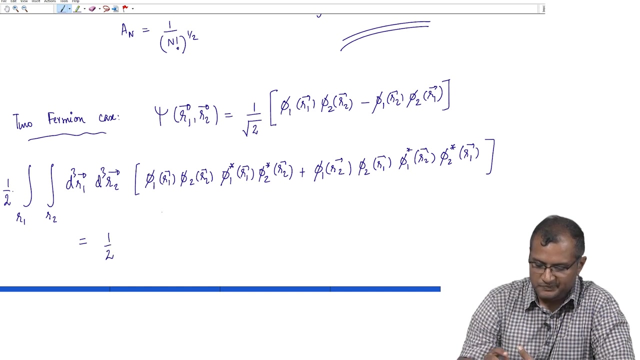 Kronecker delta function. ok, That is the. I have two terms that will basically contribute and I can write this as now: 1 upon 2.. The first term can be written as integral on R 1 d cube: R 1. phi 1. R 1 into phi 1. star. R 1 into integral R 2.. I can simply write down: 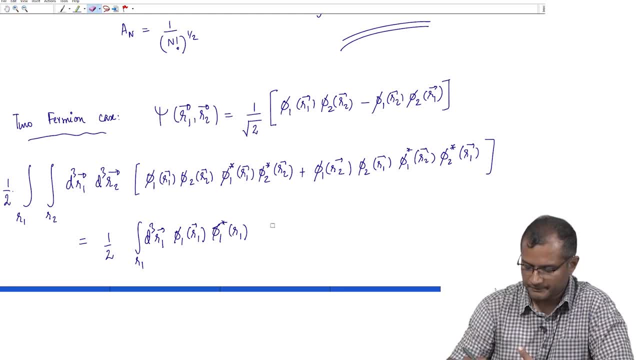 this as a. That is the integral function. we cannot call it as mandible. it is either integral of 1 upon plus 1 upon Q, R minus 1 upon square of this, because these are independent integrals. 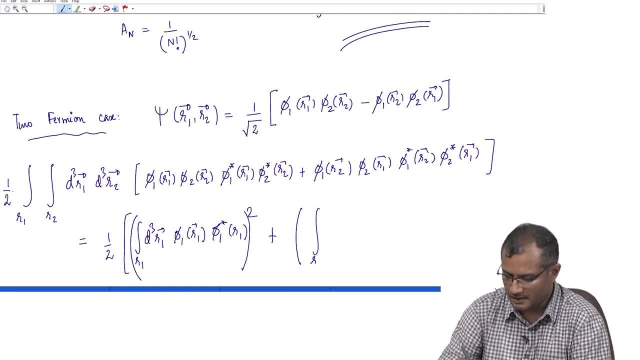 plus integral on R 1.. integral on r 2, if you want. If I want to do it in r 1, then I have to choose phi 2 here, and the other integral is basically a definite integral, the same type. So there is nothing. 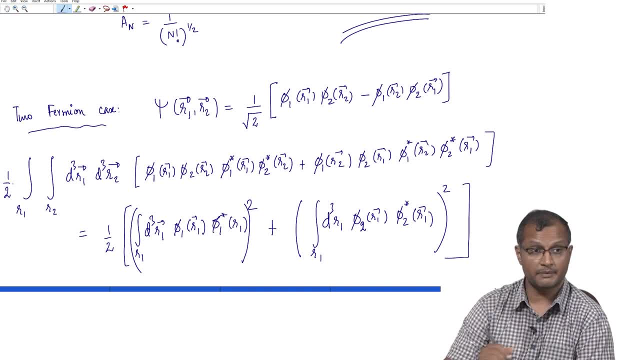 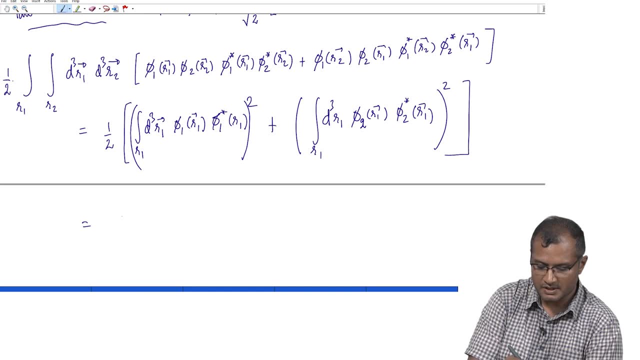 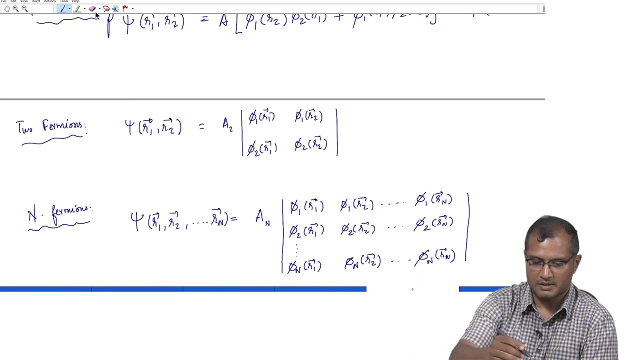 but the square of this integral, is it ok? Because r 1 and r 2 are independent, I can write a square of that which is nothing but 1, because each one of them is 1 from the orthogonality. So this is how I am going to write down the normalization prefactors. So for this, a n. 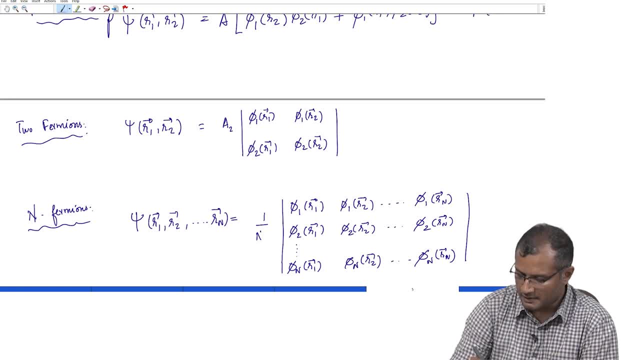 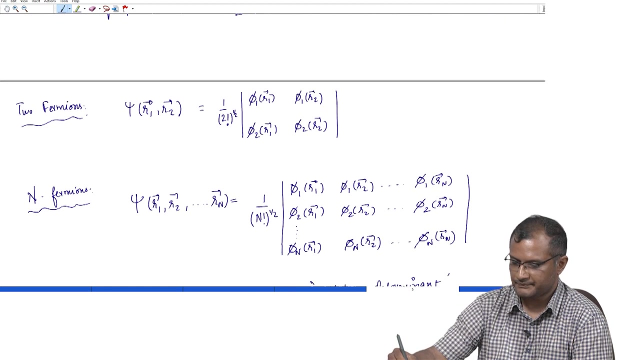 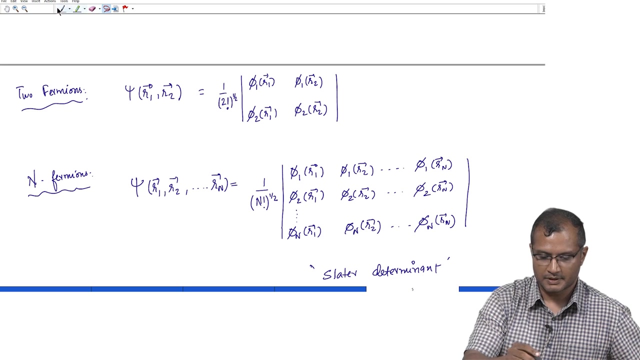 I am going to write down 1 upon n factorial square root and for a, 2, I am going to write down 1 upon 2 square root, 2 factorial. ok, So now you can see. if I just So, let me use this n particle wave function, I can see how Pauli's exclusion principle 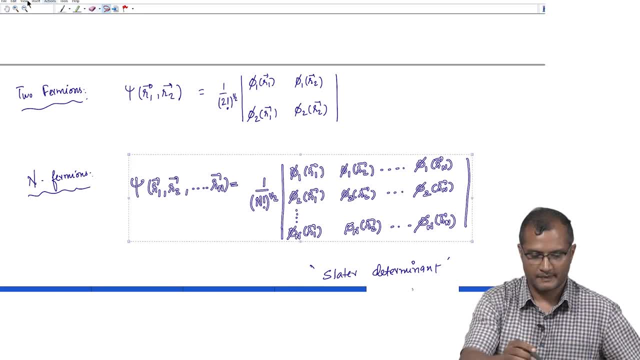 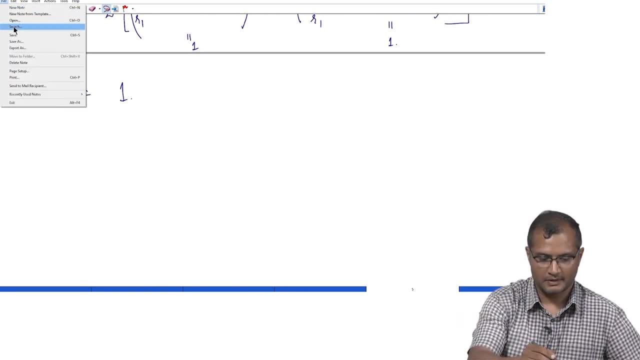 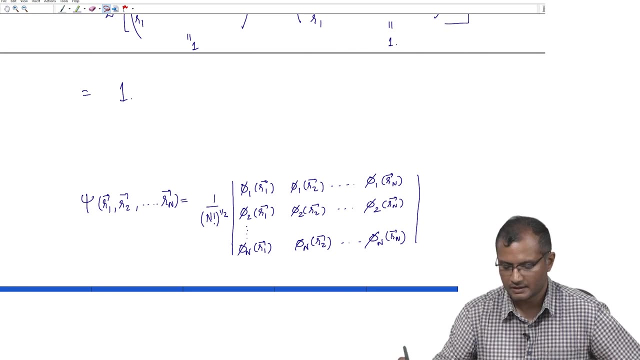 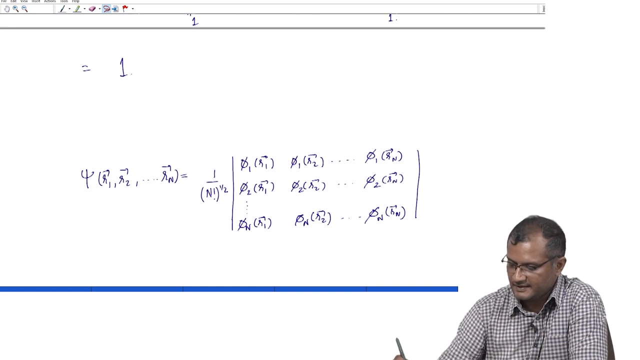 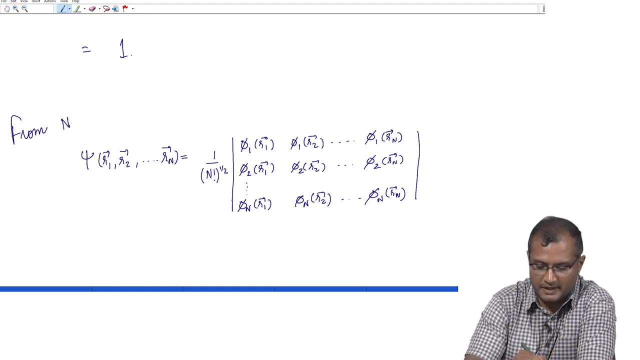 naturally arises. can you see why? Can you see why? So suppose so from this n particle wave function, which is written in the form of determinant, I can simply use a property of determinant. If two rows of a determinant become same, then 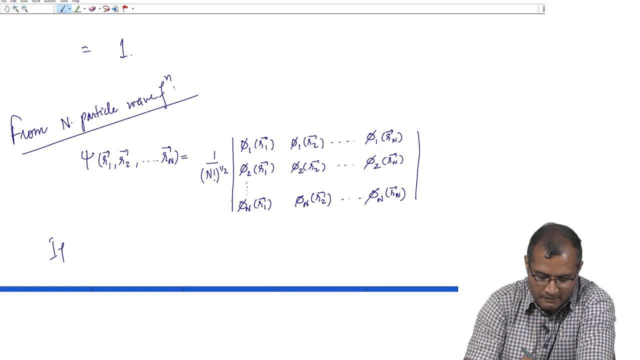 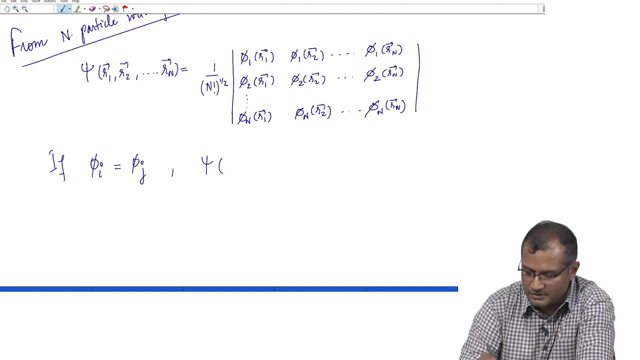 the determinant collapses. which means if some random i th row becomes the same as the j th row, Let us say phi 2 row becomes the same as the phi 3 row, then the determinant will collapse. So the n particle wave function will collapse to 0, ok. 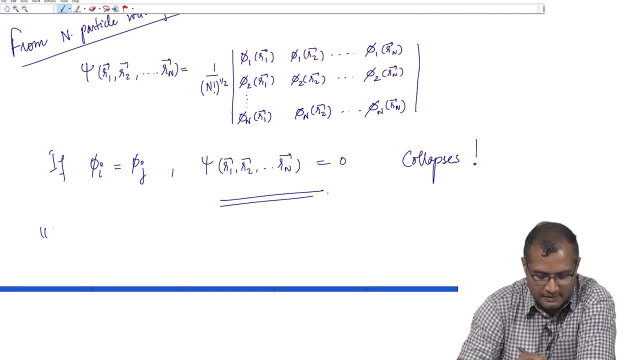 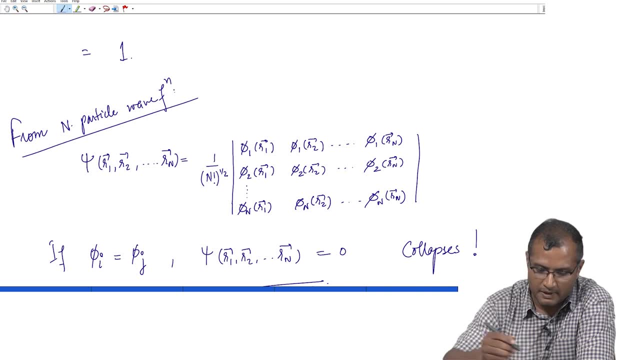 Which actually is the mathematical statement of the Pauli's exclusion principle for fermions. ok, Now I must not write down n particle wave function. I must be very specific that this later determinant is n fermionic wave function. ok, So that is the region of Pauli's. 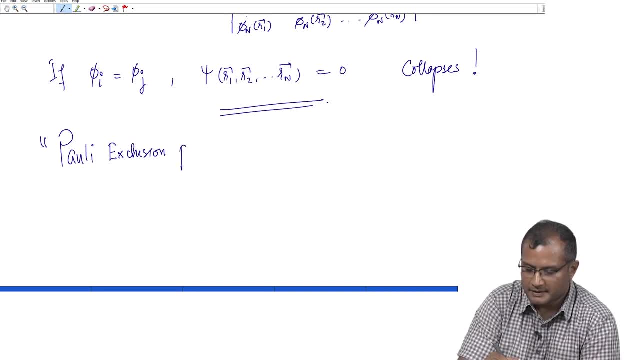 exclusion principle, So that you cannot force two fermions to occupy two identical single particle states. So if two single particle states, i and j, phi i and phi j, become the same, then the entire wave function of the system will collapse and that microstate has zero weight in your 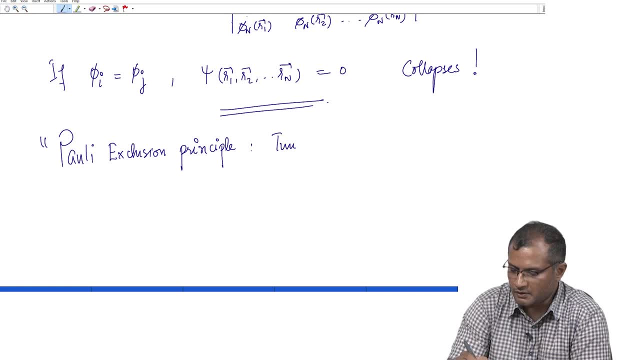 microstate: ok. Two fermions cannot occupy the same single particle state: ok. So that would be very simple because that could simply make two rows of my state of determinant identical. ok. And for example, for a two particle system, it is very simple for psi r 1, r 2, it is very